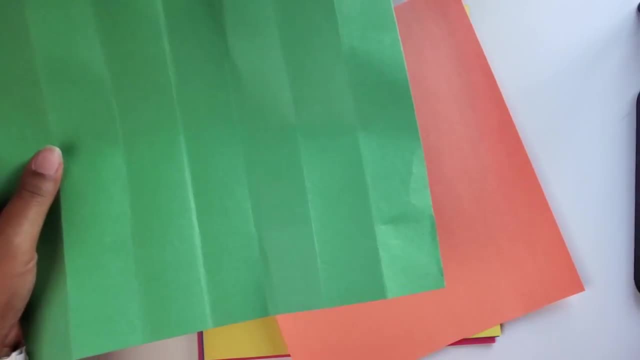 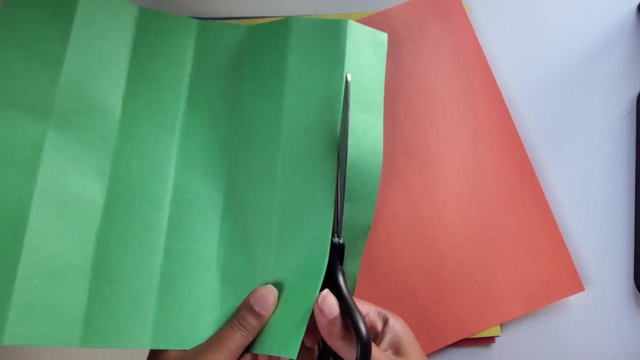 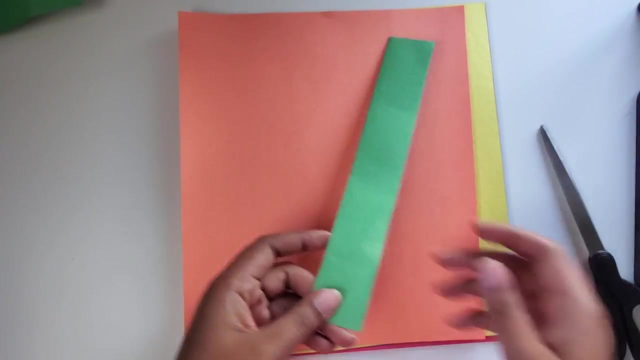 So then what you're going to do is cut one piece off, and that's going to work as your template for the other fraction- strips that you're going to create. All right, So you want it to be pretty straight. It doesn't have to be perfect, but as accurate as you can get. 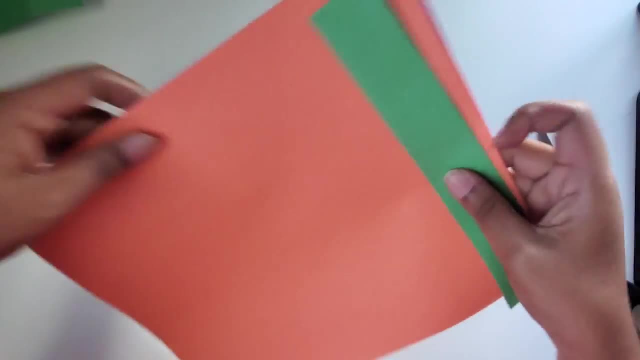 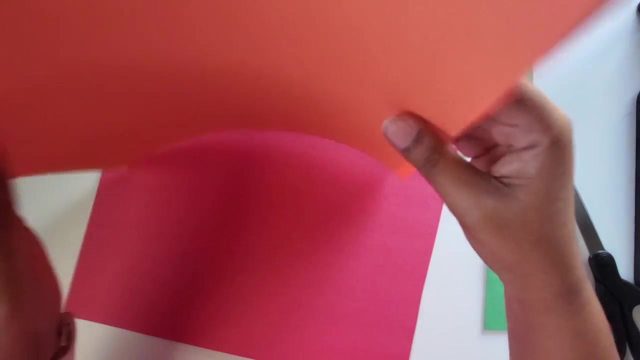 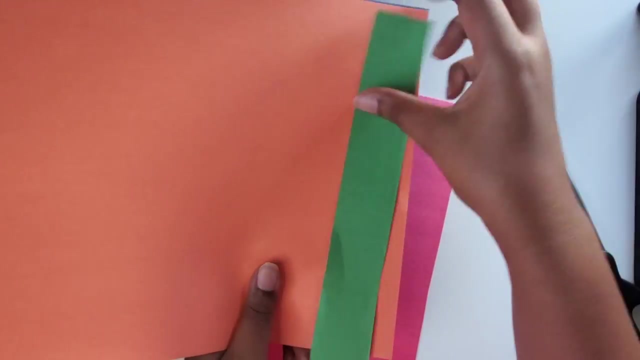 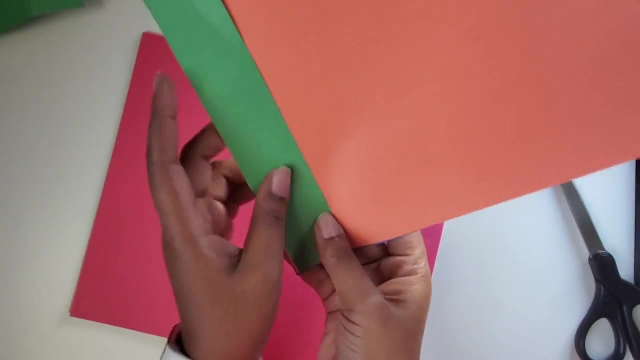 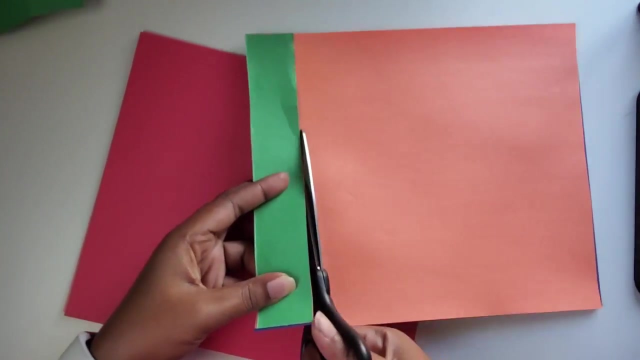 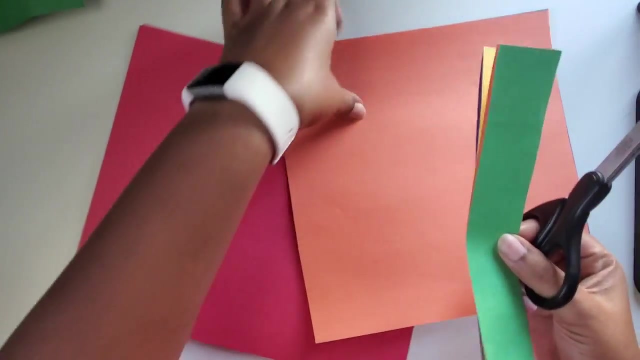 it. Then I'm going to take these other sheets of construction paper and I'm going to do three at a time and line it up with the green paper and then cut So I have all of my strips about the same size. I'm going to move that out of the way. Then I'm going to do the same thing for the next three. 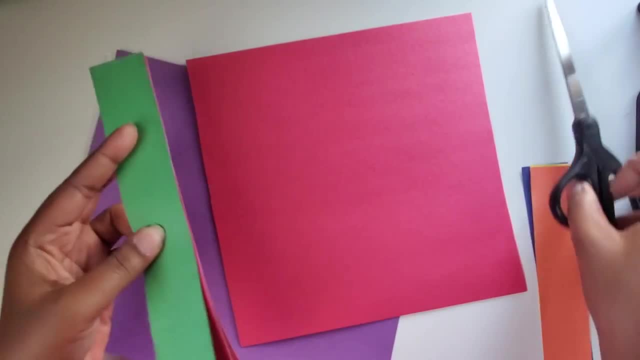 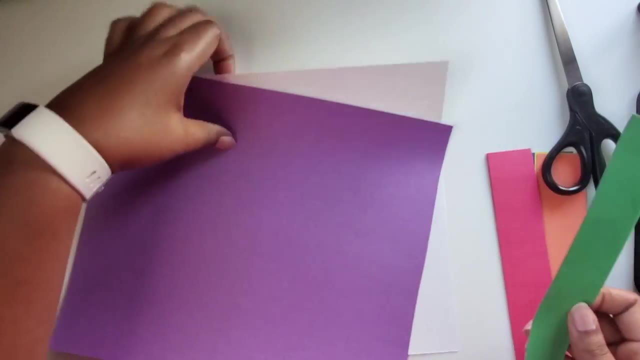 And you can also do this at school, if you have a cutting machine, or if you have your own cutting machine, Or if you have your own cutting machine at home, It'll help you go a little bit faster. And then the last two sheets. 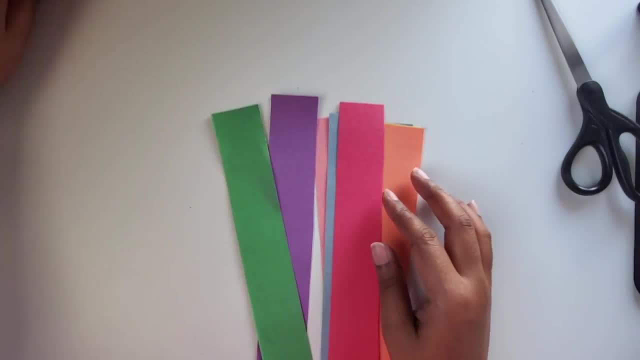 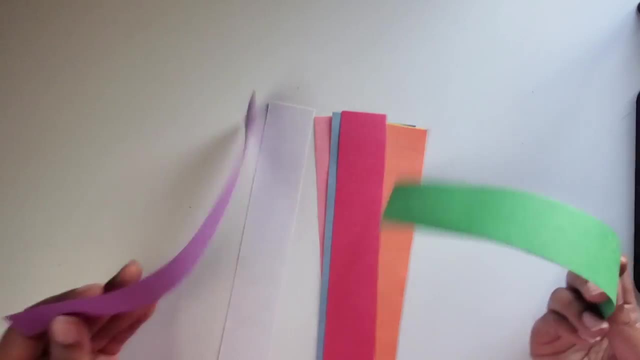 So now we have all of our fraction strips that we're going to be using to create our. Now we have all of our construction paper that we're going to be using for our kit. So now you want to design your template. Now you want to designate a color to a certain fraction value. 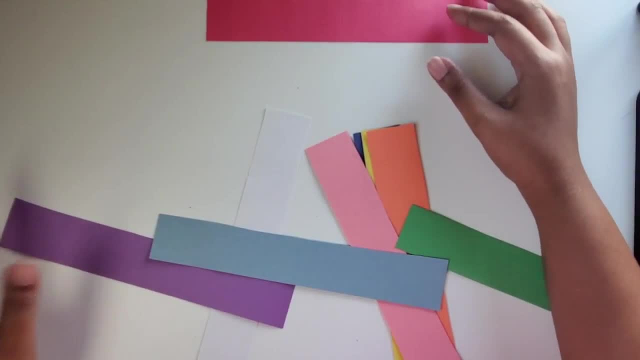 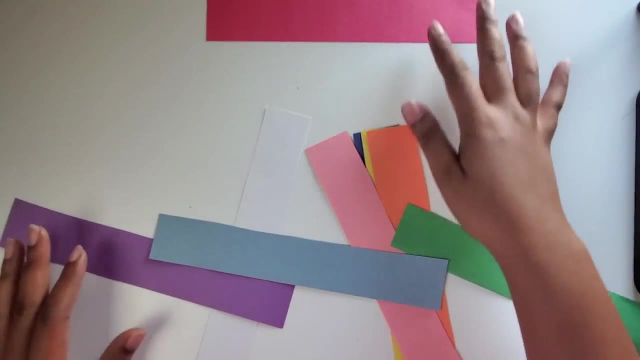 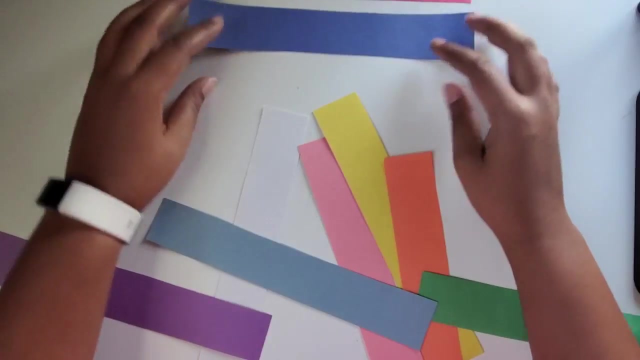 So it's going to be similar to ones you might see online or actual physical fraction tiles or strips. So we're going to use the red as the whole. We're going to use the dark blue as the halves, The pink as the thirds. 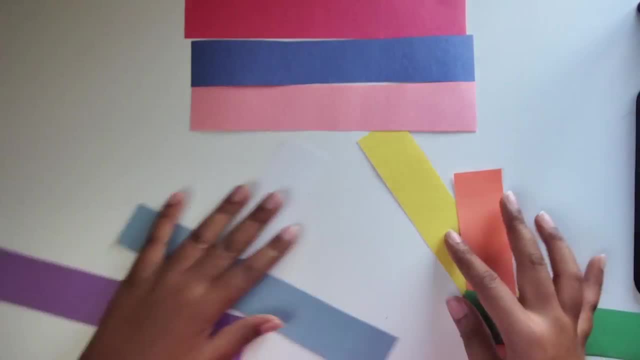 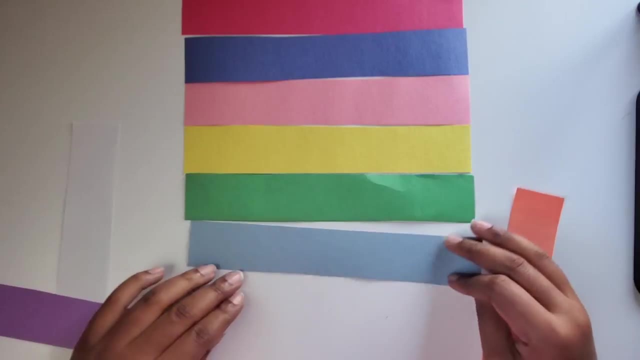 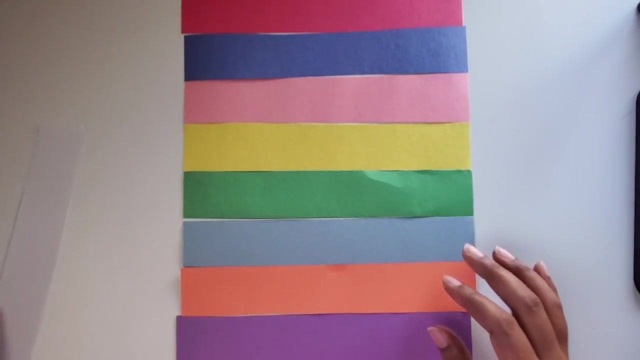 Let's see if you can see that. The yellow as the fourths, The green as the fifths, The light blue as the sixths, The orange as the eighths, I'm going to see purple for the tenths And then I'm going to use white for the twelfths. 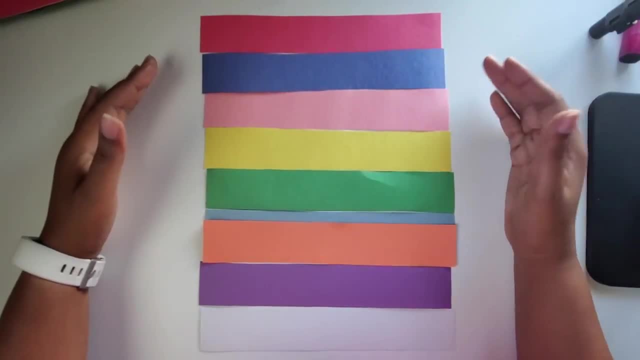 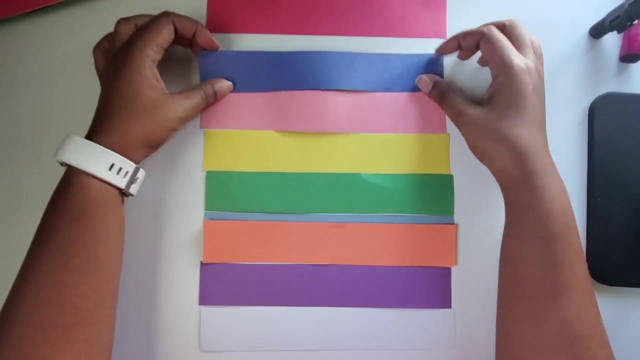 So we have our strips. What we're going to do is fold to create our fraction strips. So, because our red strip is going to represent the whole, we're going to leave that alone. We're going to take the blue strip and fold it in half to create halves. 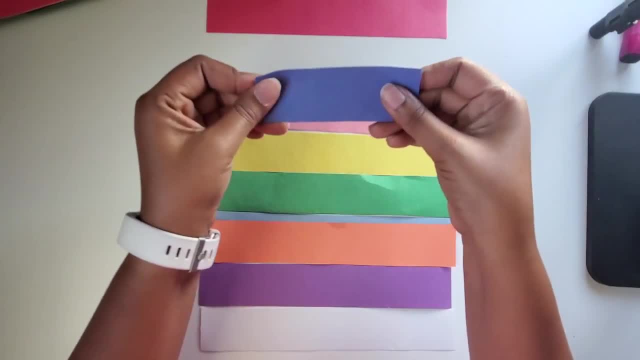 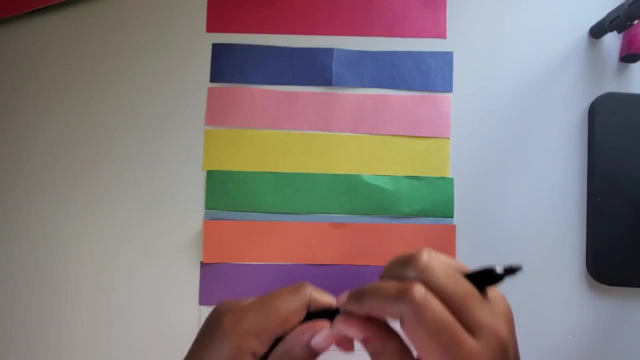 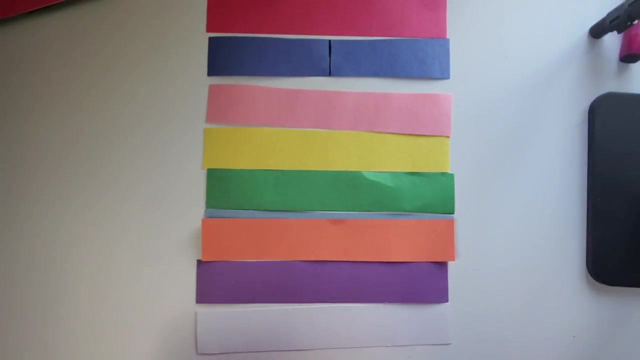 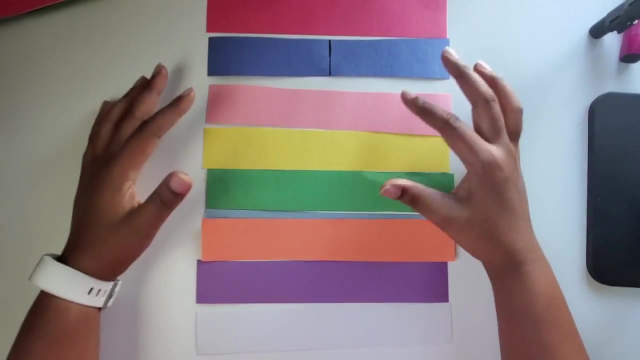 Simple, right. So what I'm going to do after I fold each strip is outline where the fold is, just to emphasize where that partition is. So we have halves. I'm not going to label them any further Because I want my students to work with fraction strips without labels. 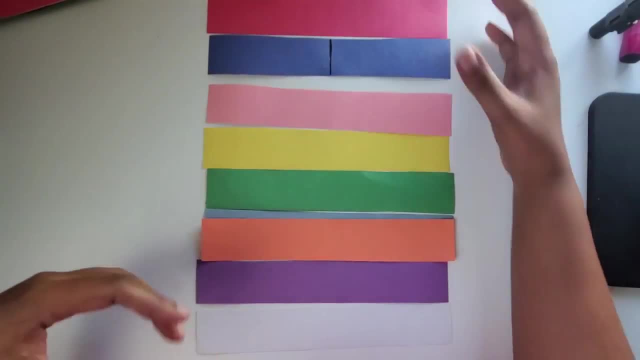 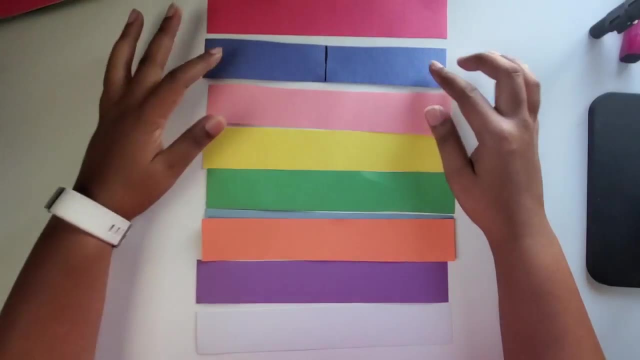 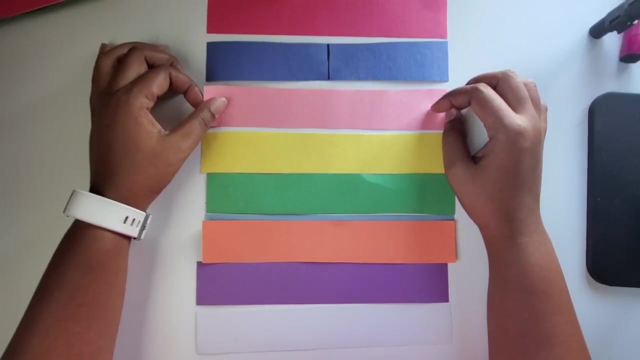 Just to show that if the whole can change, then that fraction size will be different based on whatever the whole is, But we'll talk about that in a different video. Okay, so now the next color is pink, And for this demonstration it's going to represent thirds. 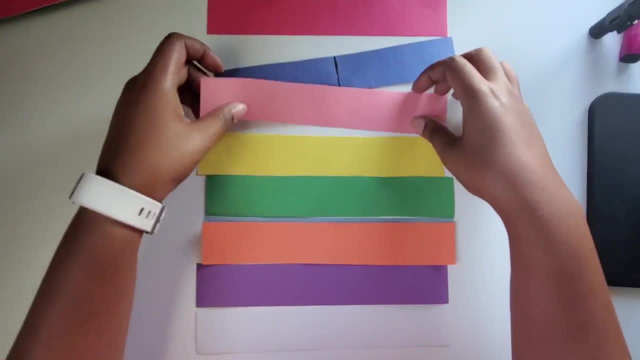 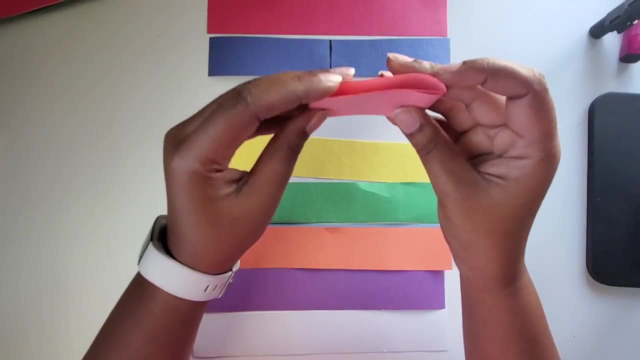 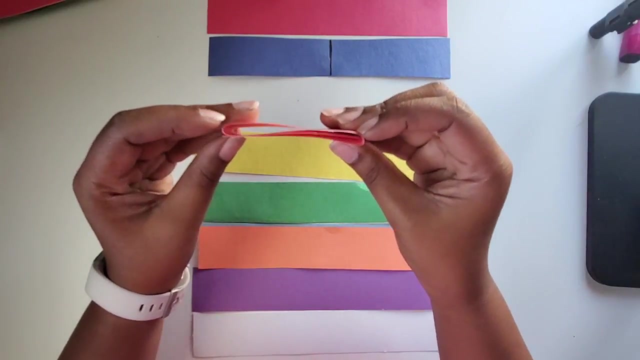 To create thirds. I kind of like to make like a little burrito, A paper burrito. if you make a lot of foldables with your students, Sometimes we use the term burrito or we say like an envelope, in a way Where you try to get most of the sections to be about the same. 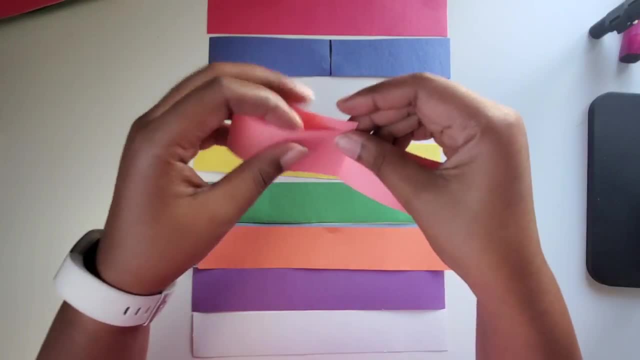 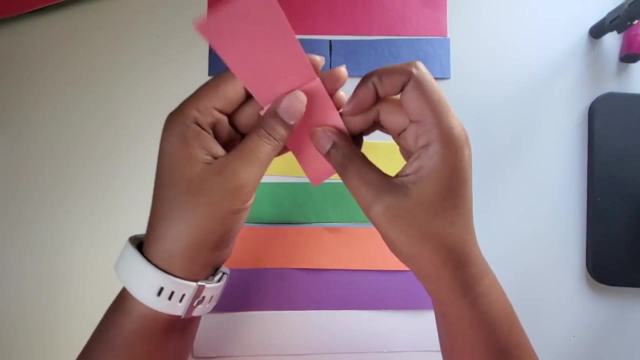 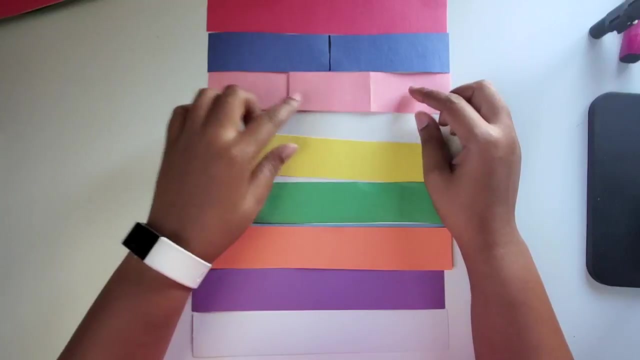 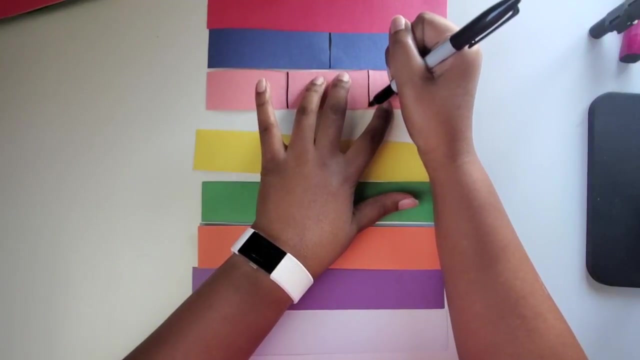 You can use a ruler if you want, But I try to estimate it with my eyes. So they're generally It is. Each third is about the same, So I'm going to outline that. Now we're going to use the yellow strip to create fourths. 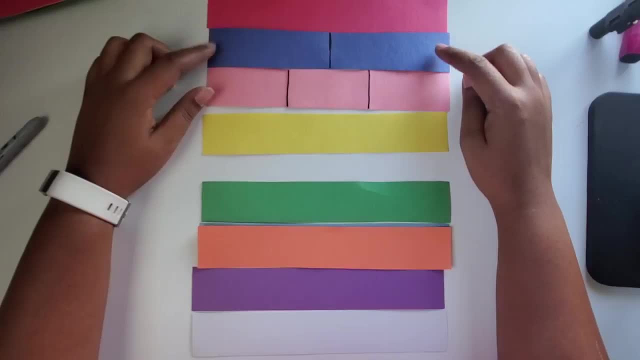 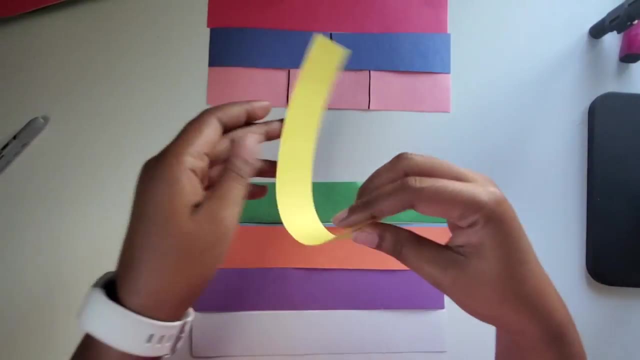 So the great thing about fourths is all you need to do is make your halves And then partition or fold those halves in half And it will create fourths. So we're going to fold our strips, We're going to cut our strip in half. 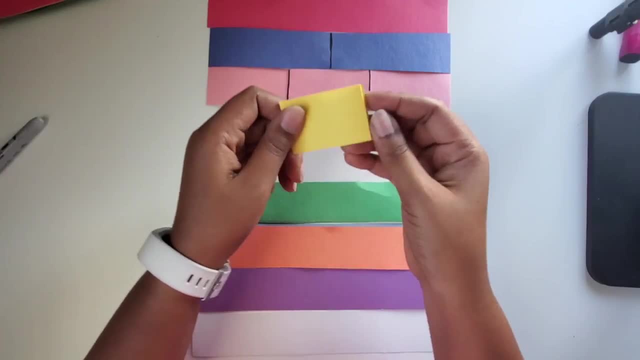 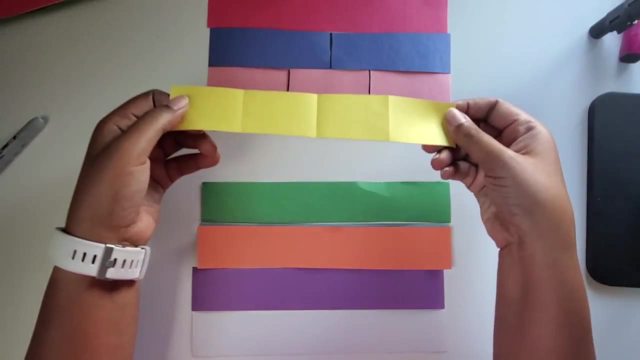 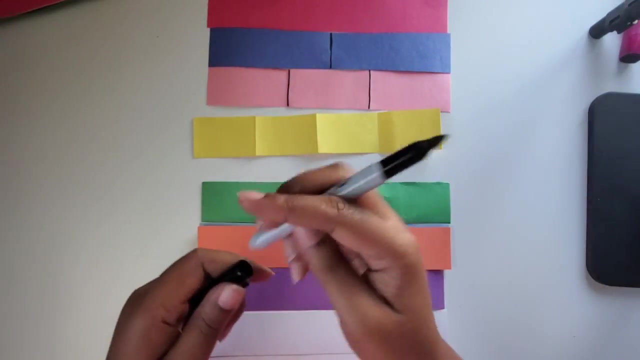 And then we're going to fold it again to make fourths. And they are fourths because it takes four of them to make up that whole piece. So I'm going to fold these one more time And then outline where the folds are. 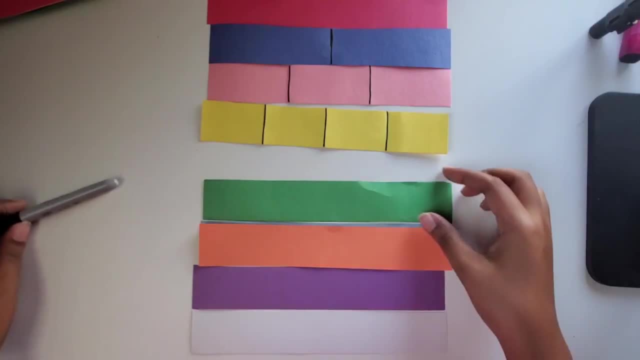 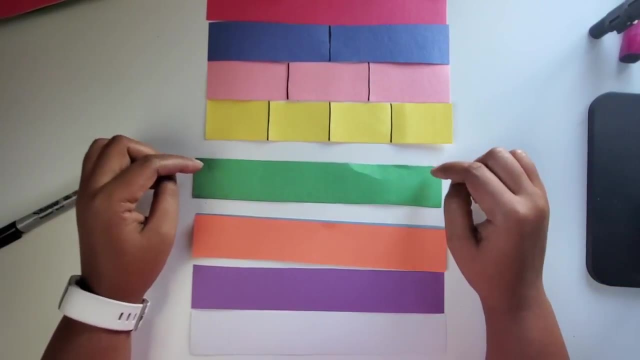 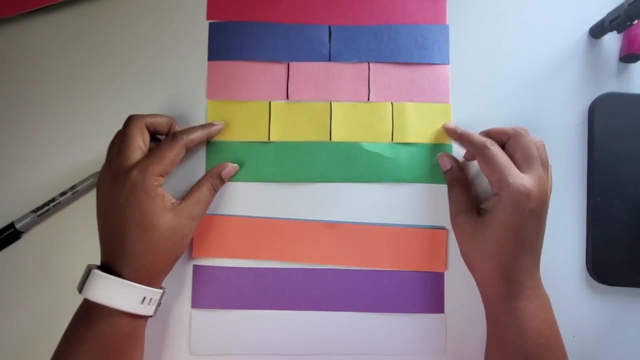 Next are the fifths. Now the fifths can be even trickier than the thirds. One trick I use to create fifths is to use the fourths. to help me, I take I line up the fifths, or what I'm going to use to make the fifths with the fourths. 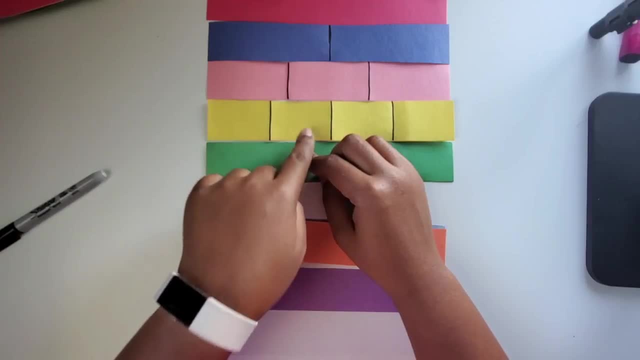 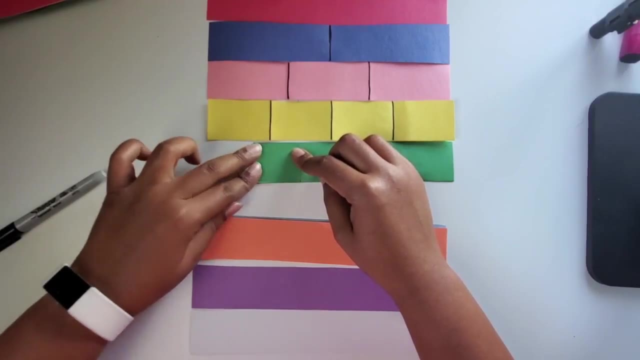 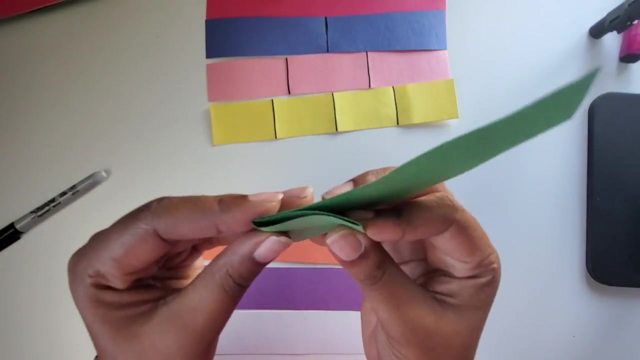 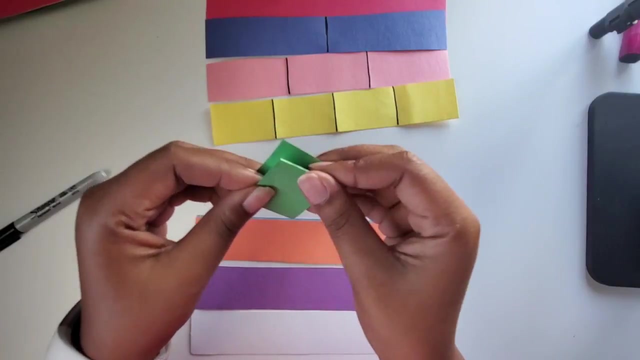 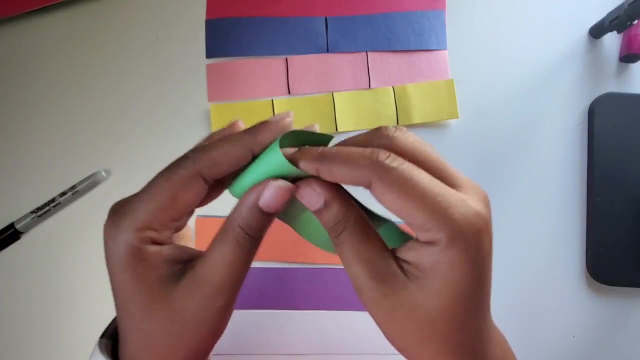 And I'm going to fold in the end to the middle of that second fourth And it creates a fifth for me. So then I just fold that in Five times- Or it's probably four times, And that creates my fifths- And then fold on the back side. 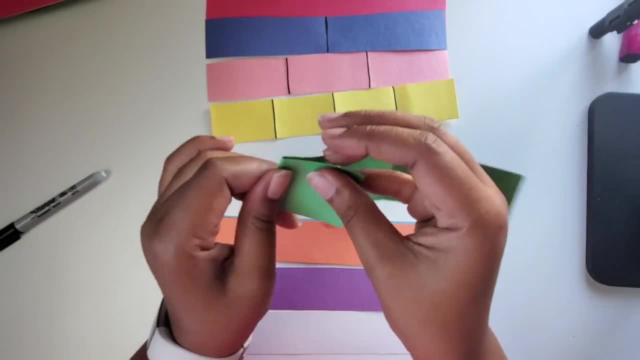 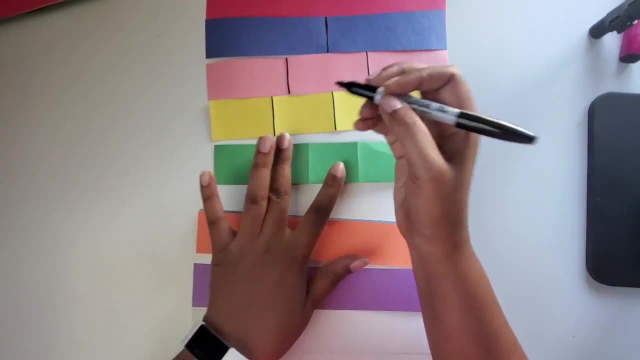 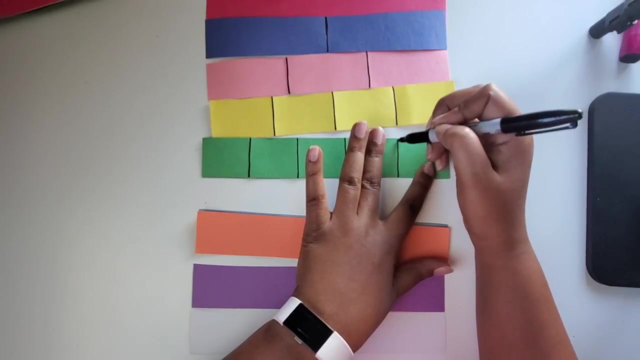 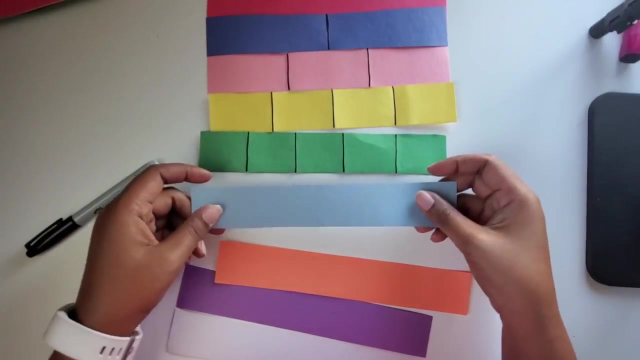 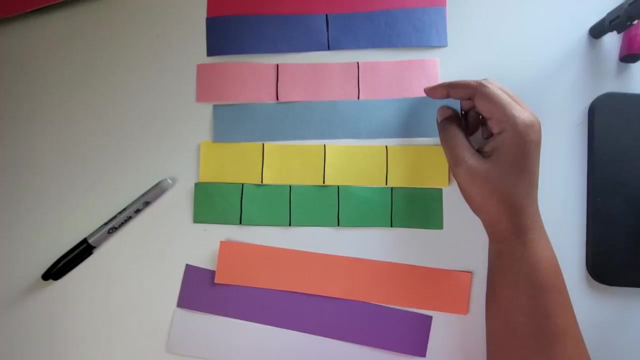 Just to reinforce those fold marks, Alright, And then we're going to outline: Okay, Next we have our blue strips to create our sixths. So sixths are just the thirds. And then we're going to fold those thirds in half to create sixths. 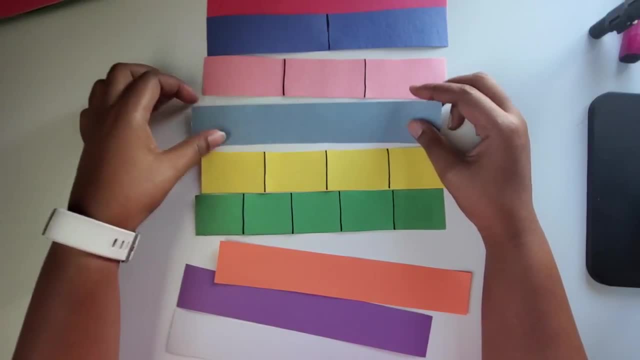 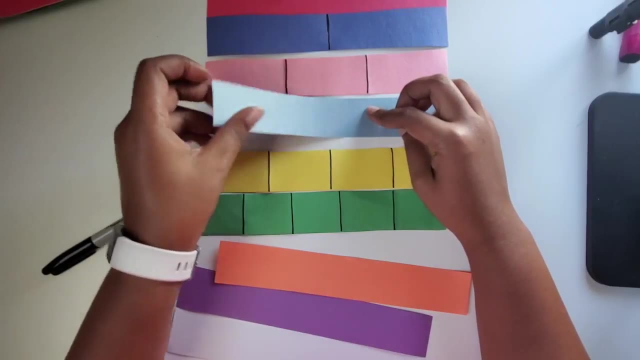 Just like what we did. We did with the fourths. We started with the halves And then we folded them again to make fourths. So I'm going to use the thirds as a marker And just fold in to where the third. 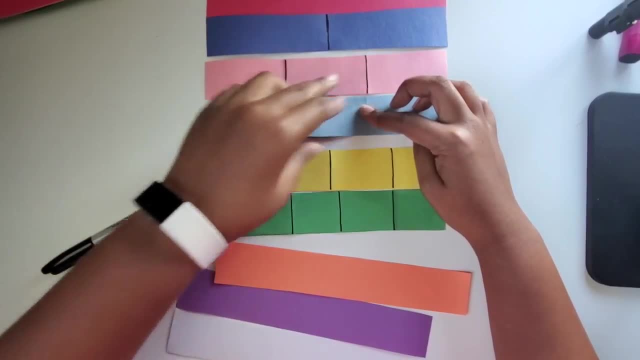 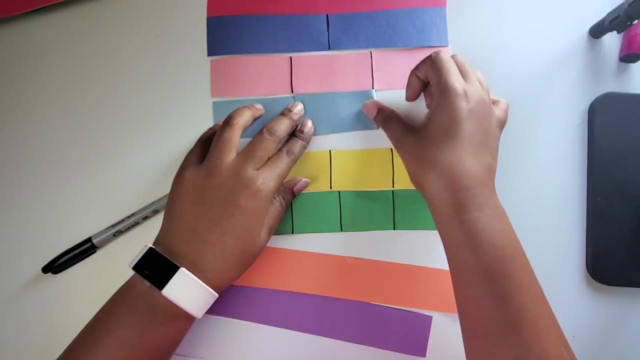 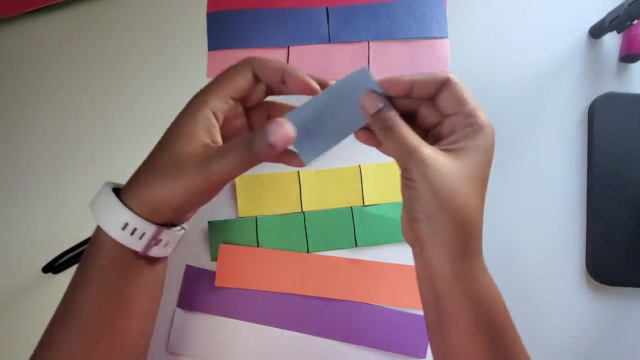 To where it stops, Instead of making that burrito shape A burrito style. A burrito is not a shape. So there I have my thirds, So I'm going to fold them in, And then I'm just going to fold that third size piece in half. 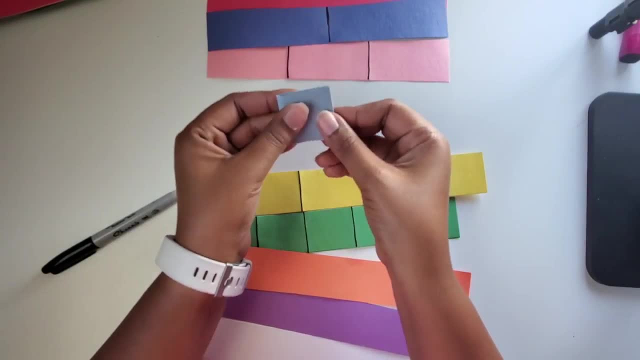 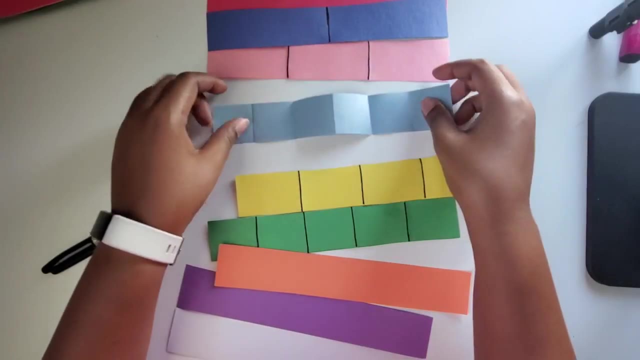 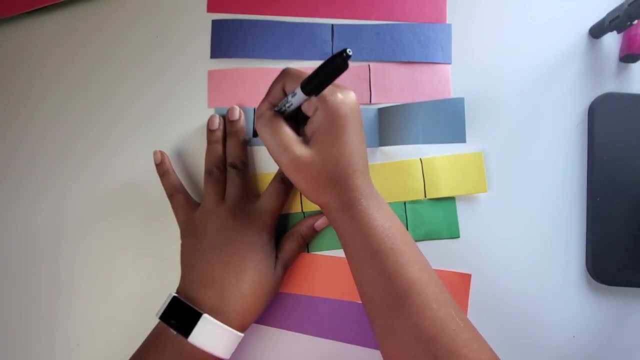 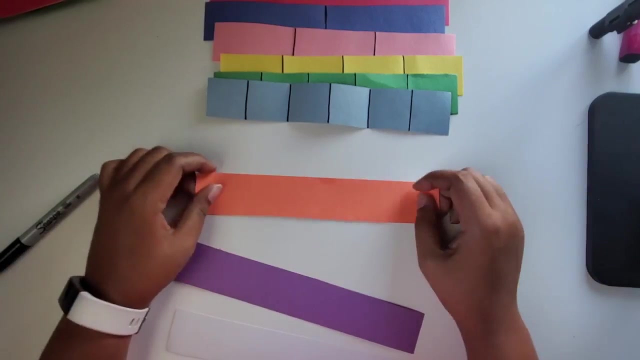 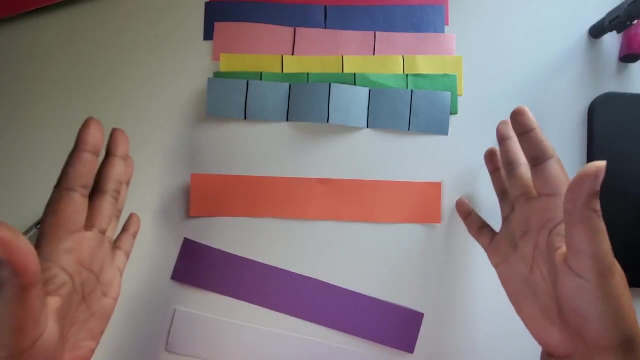 Or in two, And that creates six size fractions. And they are six because it takes six of them to make that whole. So we're going to outline our six size fraction pieces Now we're going to create eighths. So our eighths fall right in line with our halves and our fourths. 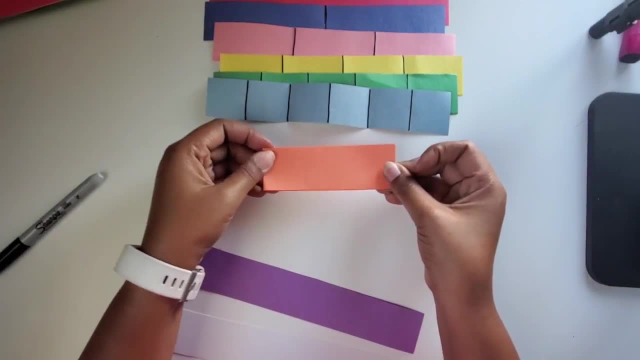 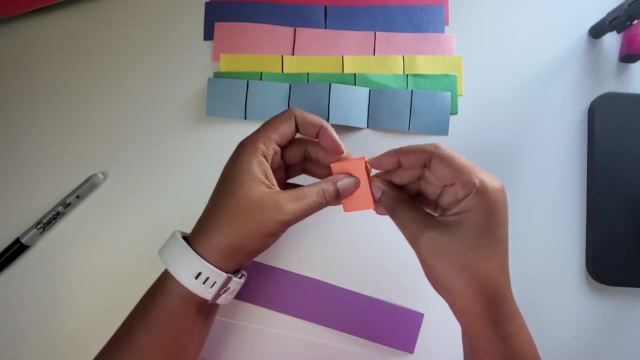 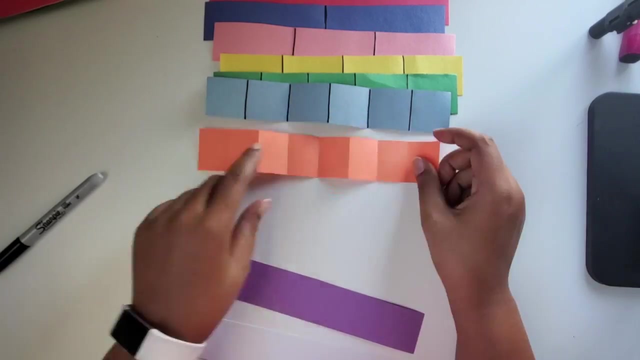 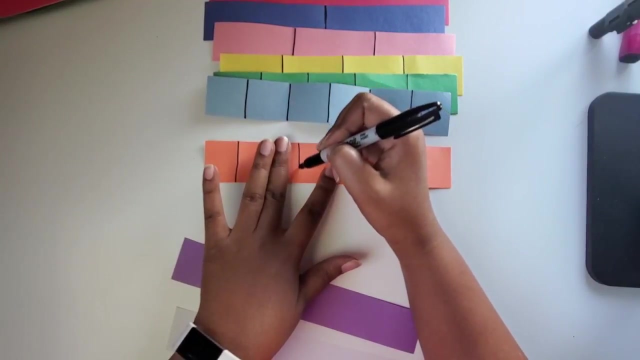 So I'm going to start by making halves. Fold that, Then fold it again to make fourths, Then I'm going to fold it one more time to make eighths. This is great to do with your students when you're exploring fractions in second or third grade. 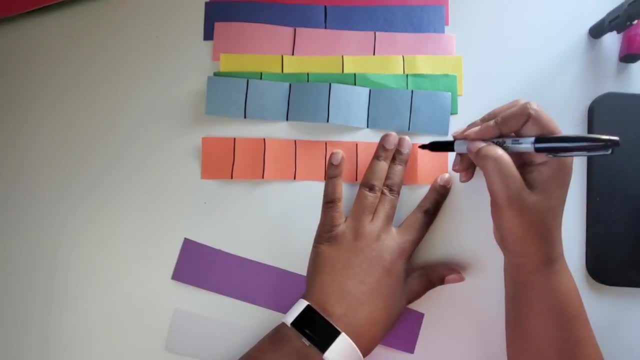 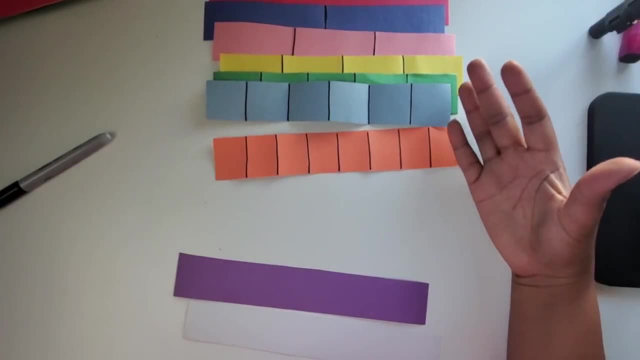 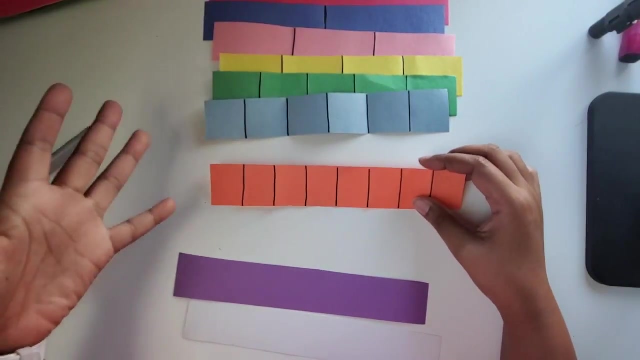 Or reviewing in fourth grade When discussing equivalent fractions or comparing fractions as well. And then you can use the fraction strips to help with adding and subtracting fractions later on, After they understand the foundations of fractions. So we have our eighths. 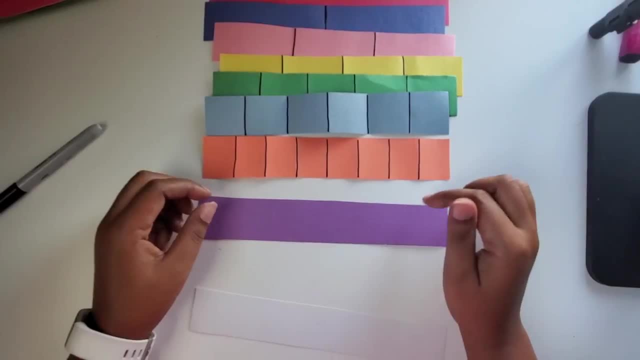 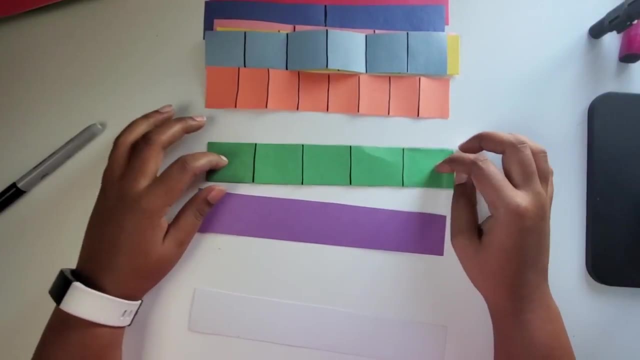 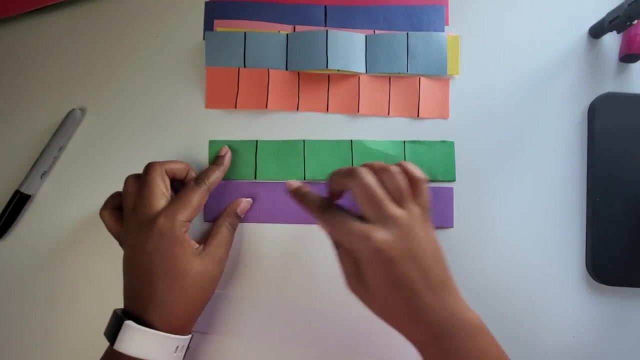 Now we're going to use the purple strip to make tenths. Tenths are like fifths And then fifths folded in half. So I'm going to use the fifths fraction strip as my template And just fold in. You can also draw lines there. 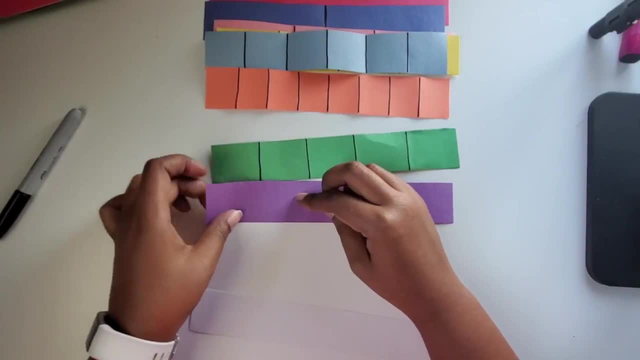 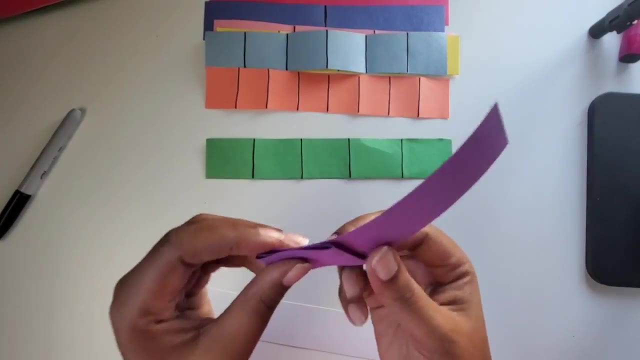 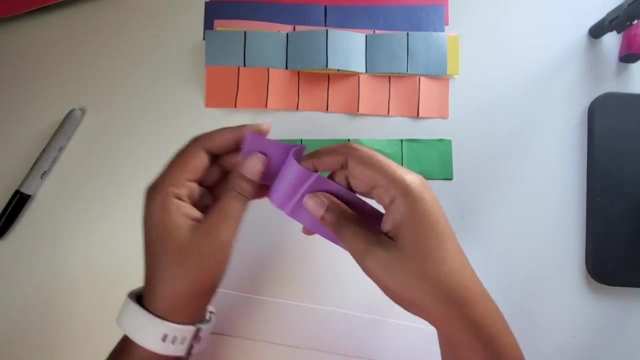 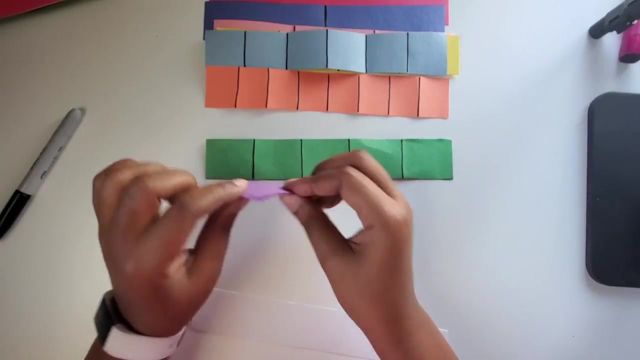 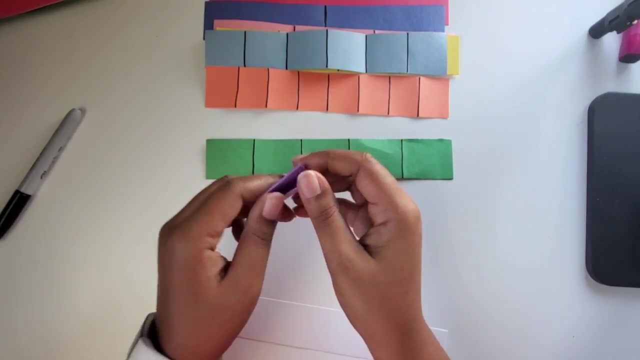 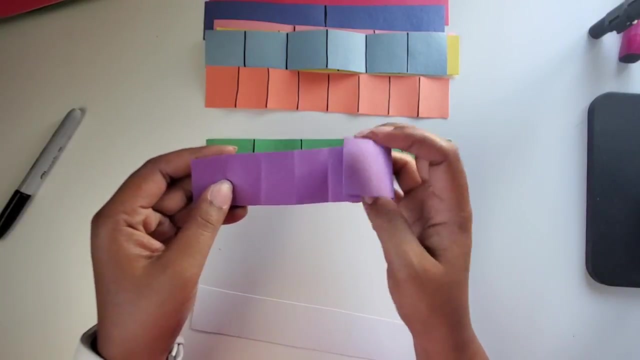 But I want to make sure I have the folds in place. So we have our fifths to make tenths. We're just going to fold the fifths in half to double our pieces. So each fifth was partitioned into two parts. So we have double our amount. 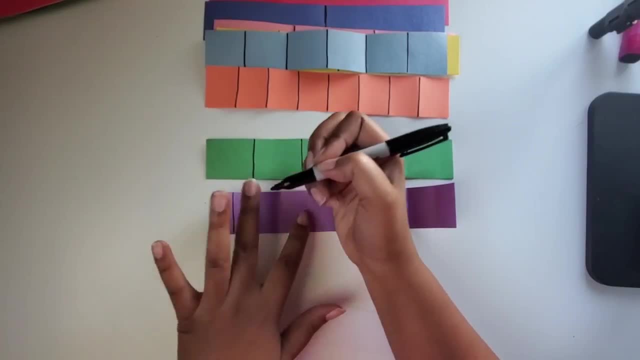 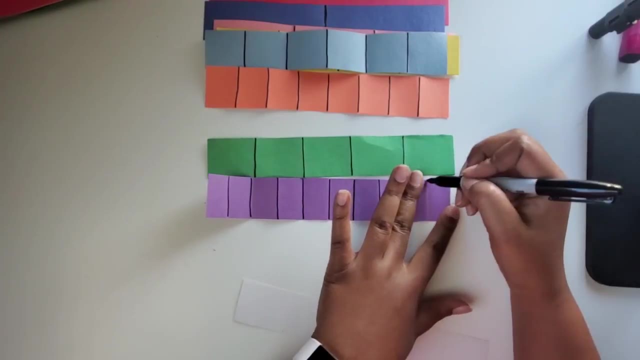 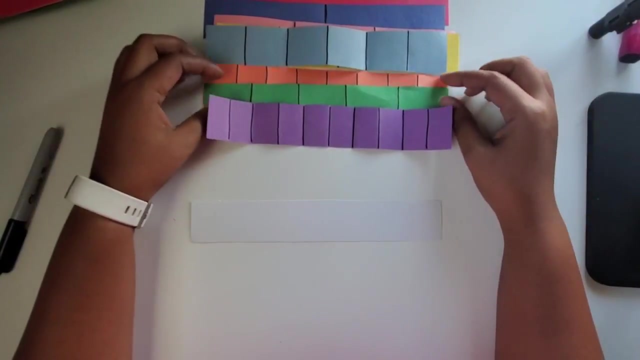 And then we're going to make our sixths, And then we're going to make our twelfths, And then we're going to make our twelfths And then, last, we're going to do our twelfths, Which is just our sixths. 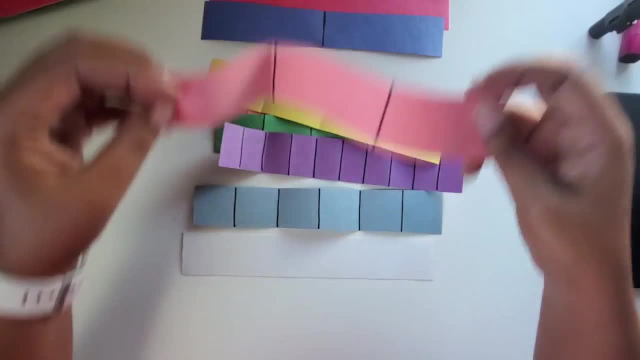 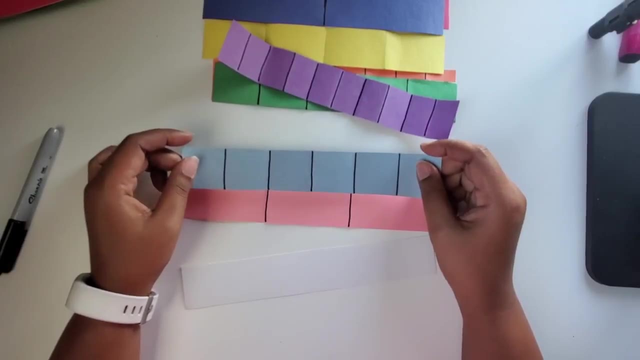 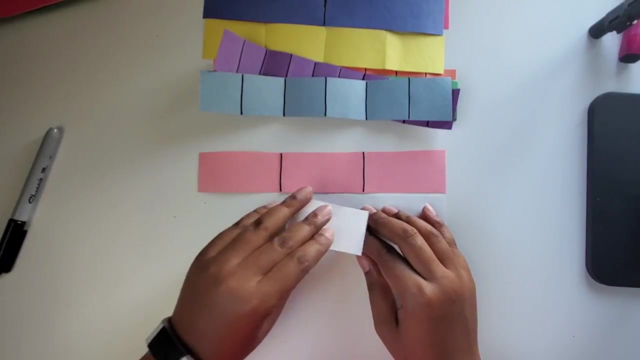 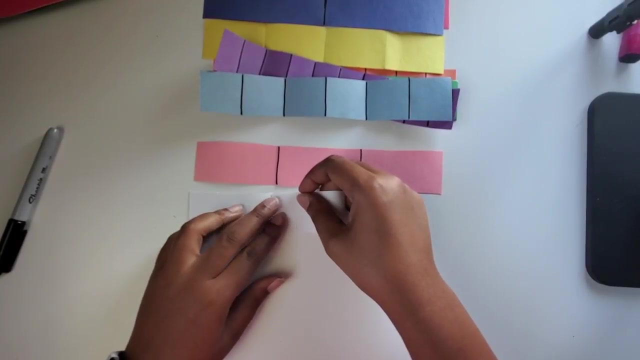 And our thirds folded three times. So we can take our sixths and then partition our sixths in half, partition our six in half or use our third. So I'm going to use the third to fold it in to create thirds and then we're going to create six, So we have our. 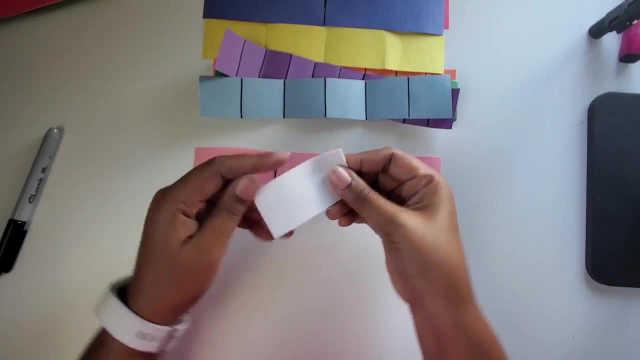 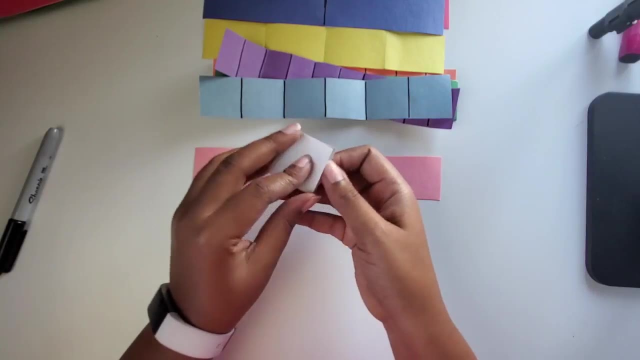 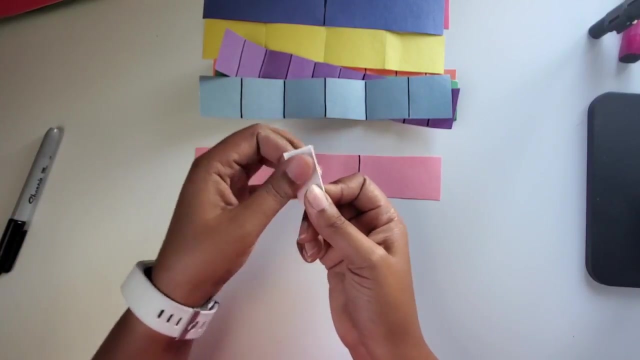 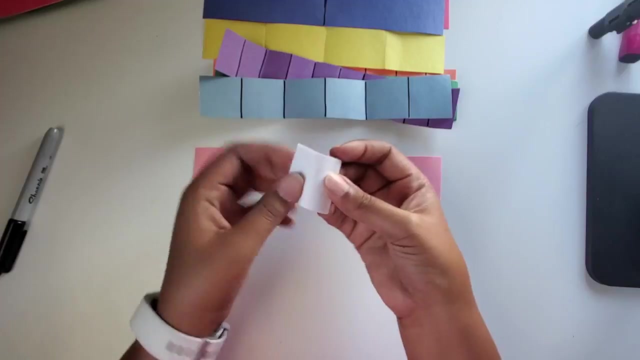 third size pieces. We fold those in half. Now we have our sixth size fraction pieces, So I'm going to fold those one more time to create our twelve size pieces, And doing this can help the students really see, even though that number is increasing, what's happening to the size of the pieces They're getting. 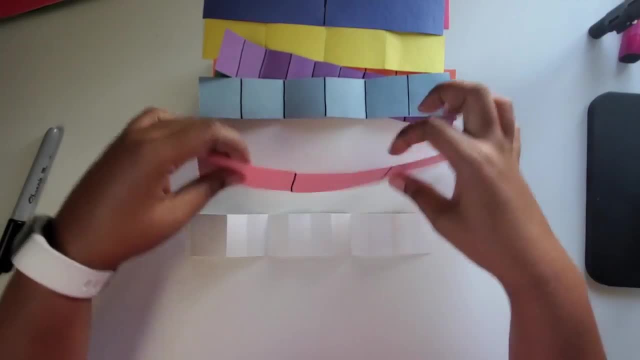 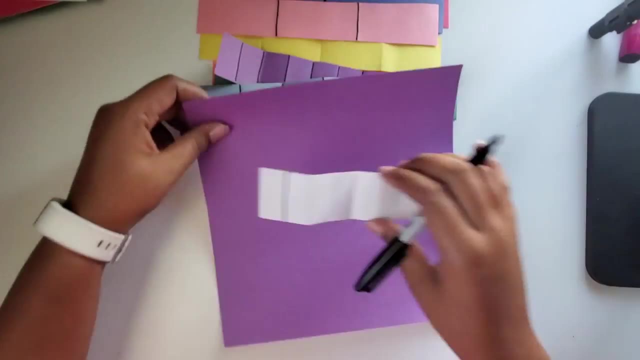 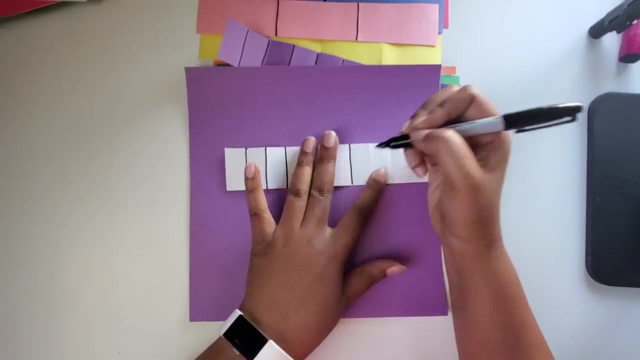 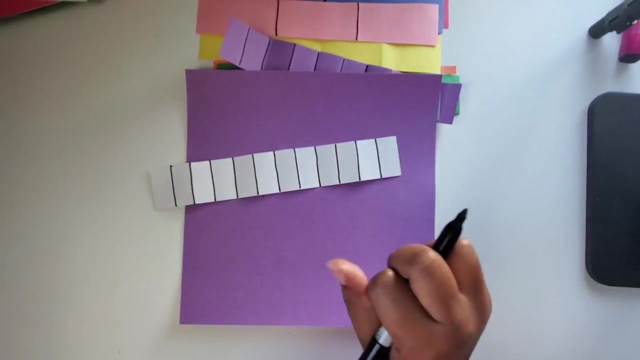 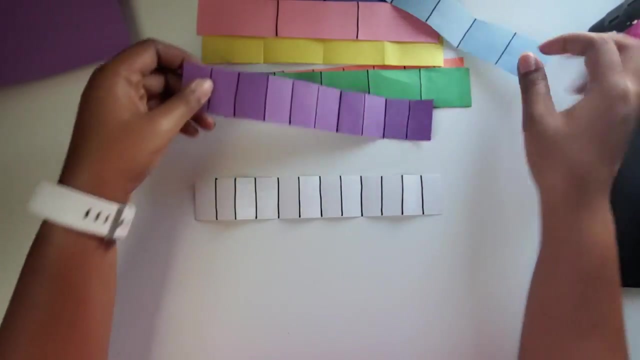 smaller and we need more of them to make that whole. So the last thing we need to do is outline our folds- Music, And there you have our twelves, Twelfths. so we have our twelfths, our tenths, our 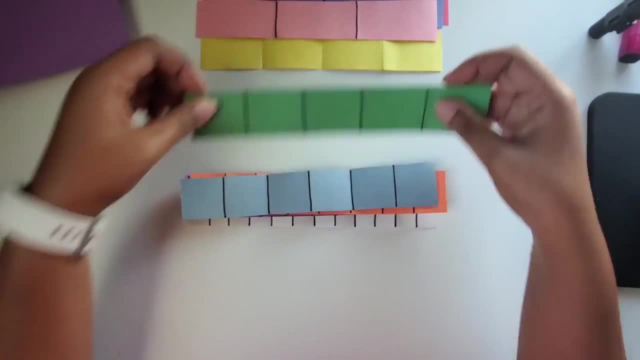 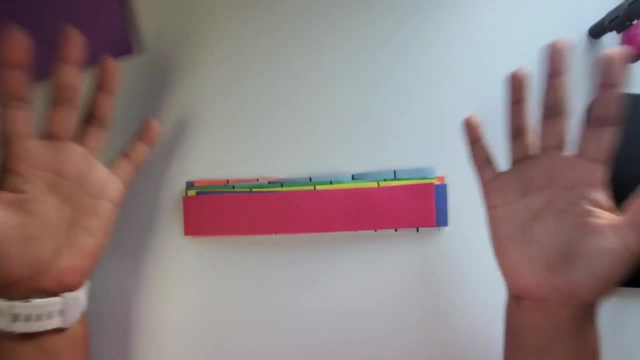 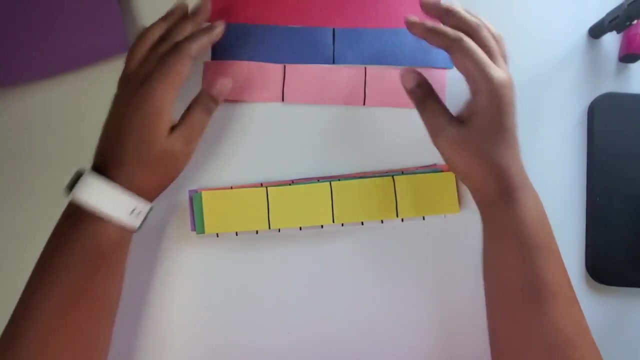 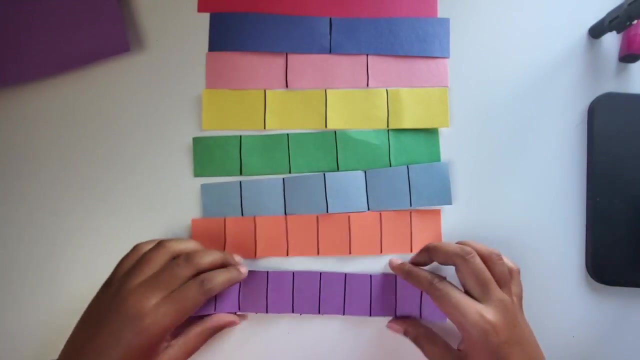 eighths, our sixth, our fifth, Music, our fourths, our thirds, our halves and our whole. So we have created our own fraction strips to work on fraction concepts in our classroom or, even better, at home with our young kids as they are learning the concepts of fractions. 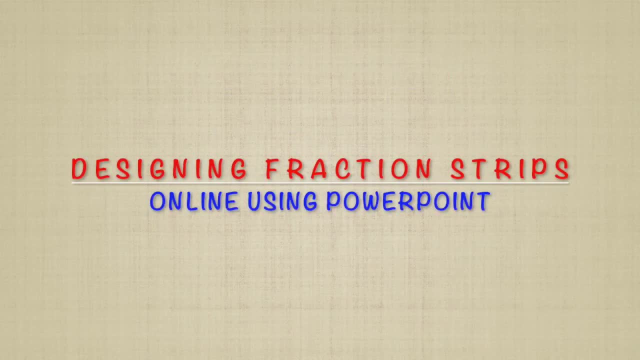 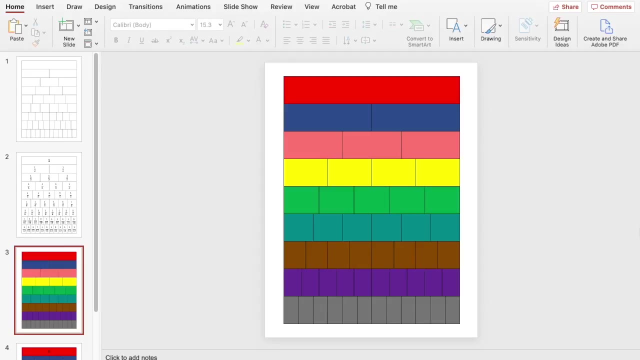 I'm going to show you how to create your very own printable fraction strips using PowerPoint. So this is the end result of what we're going to create today. So we have four slides. We have our color fraction strips with no labels. the same with labels. 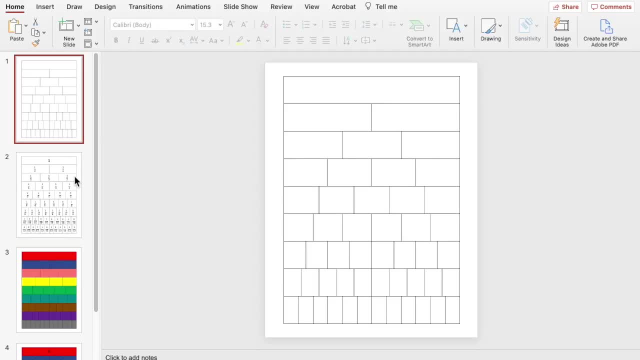 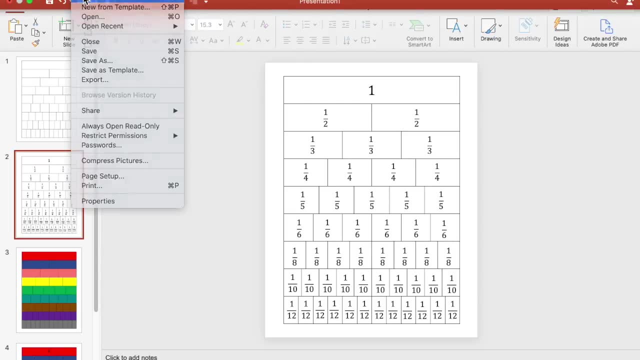 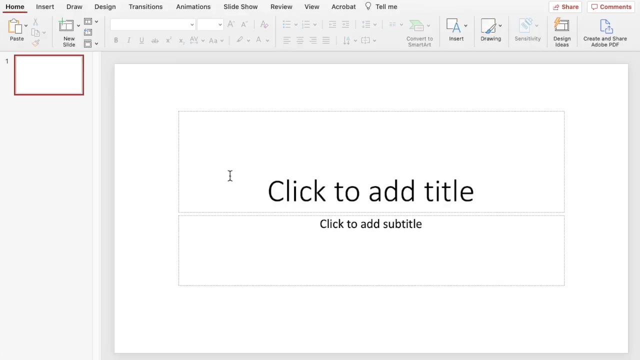 and then we have our color fraction strips and both of those without color, So they are like black lines. All right, so in order to do this, we're going to open up a new presentation And we are going to reformat our slide. 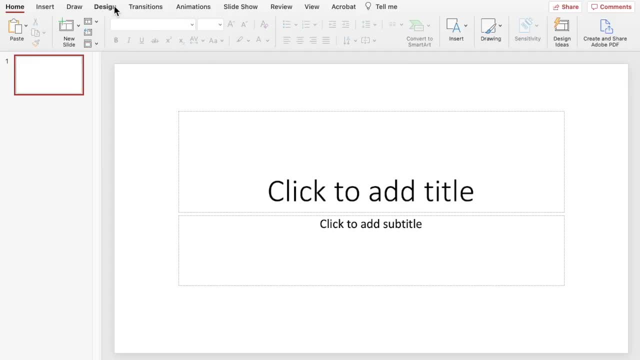 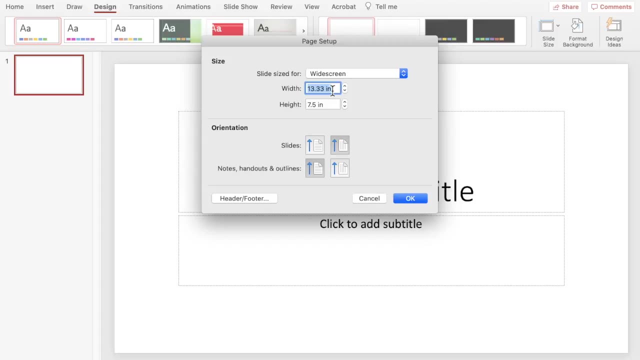 to mimic that of our printable sheet. So we're going to go to design, then over to slide size. page setup: We're going to change our width to eight points, We're going to change our height to five and our height to 11.. 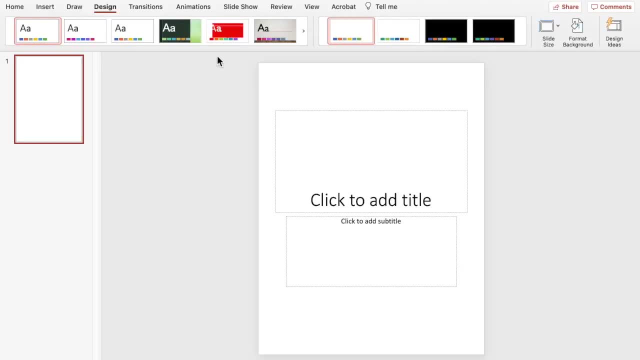 Then I'm going to hit scale up. What I'm going to do now is select the entire page and then delete the text boxes that were defaulted on the page. So now I'm going to create the fraction strips template. So I'm going to go over to insert and click on table. 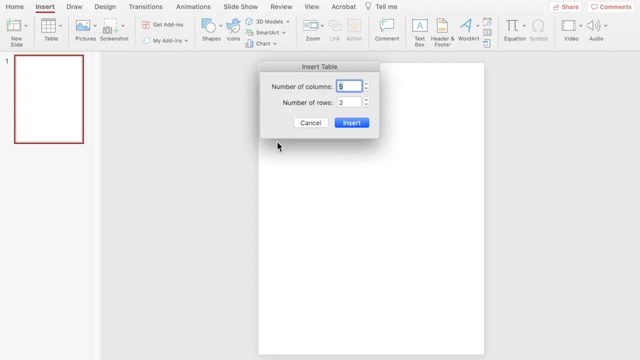 and hit insert table at the bottom. So we're going to have one and then we're going to go to column, But the number of rows is going to be nine. We're going from one whole to 12, but we won't have seventh and we won't have ninth. 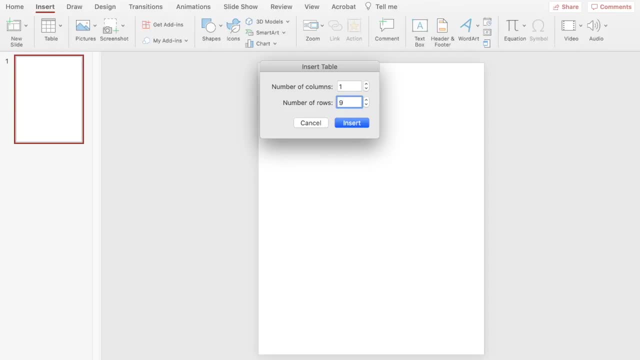 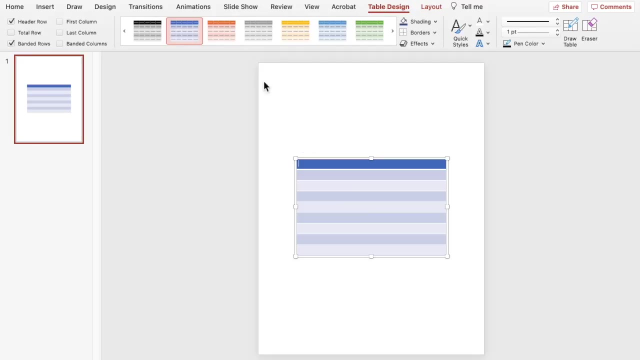 or we won't have 11.. So that's why we won't need 12 rows, So we're going to need nine rows, So we're going to insert, and there is your basic table. We need to make a few changes before we start creating our fraction strips. 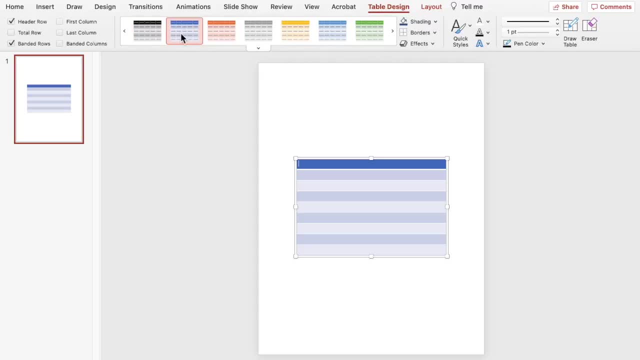 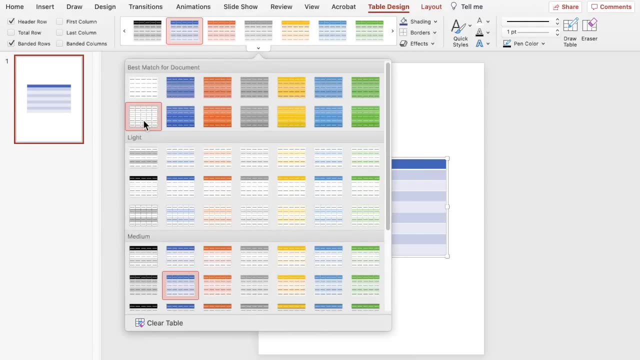 We're going to go up here to our ribbon where it has a variety of choices for your table, And I'm going to hit this drop down bar or drop down menu and then come over to light. or it says best match for document. Basically, you want to click on the one that has no style. 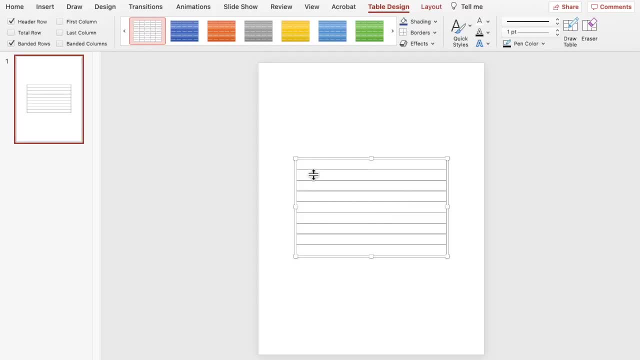 We don't want any color and no style. So now that we took away the color and it doesn't have a specific heading or style, I'm going to select it again and then go up back to the ribbon and click on layout And then I'm going to come over here to the table. row height. 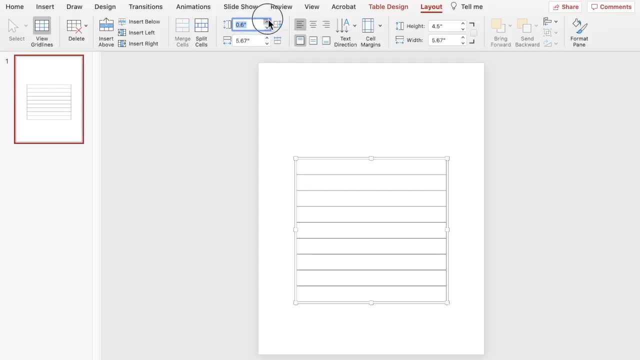 and the table column width. So I'm going to increase both. So I'm going to increase the height to one And that looks about right. Let's see if we can go up one more, What that would look like. I think that works as far as the height. 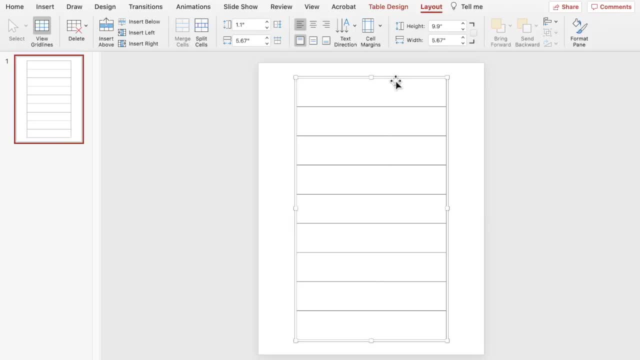 You want to remember about when you're printing it. I don't like my designs to be too close to the edge, just in case it might come off when it prints out. And then we're going to adjust the width. And the same thing when it comes to the width. 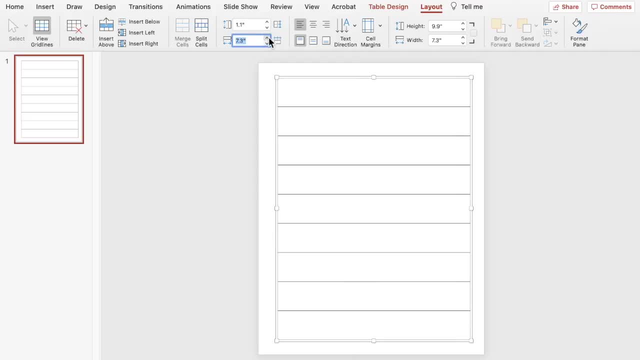 I don't want it to be too close to the edge. Let's see if we can get to 7.5.. What would that look like? All right, that works for me. So I clicked away from that ribbon. So now I'm back on the page. 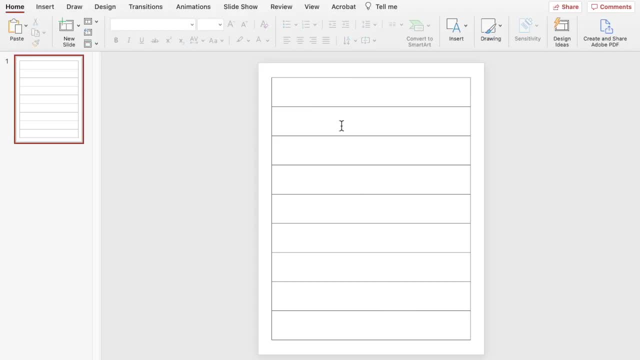 So here is the basic template for our fraction strips. So now what we're going to do is select our table. When you select that table, different things change in the ribbon, But what you want to make sure you're under is table or not. table design layout. 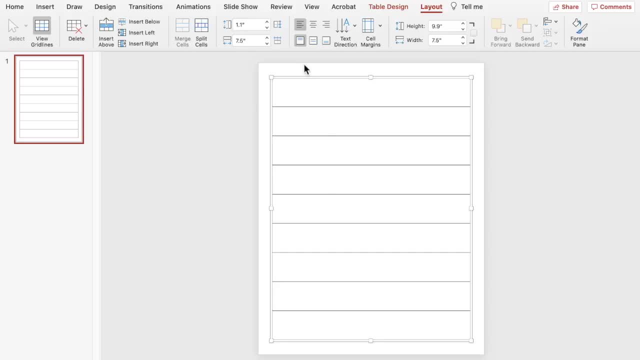 So in layout is where you can split and merge your cells. So each row in the table is a cell. So the first row we're going to leave exactly how it is, because that's going to represent our whole. The second row, I'm going to split the cell. 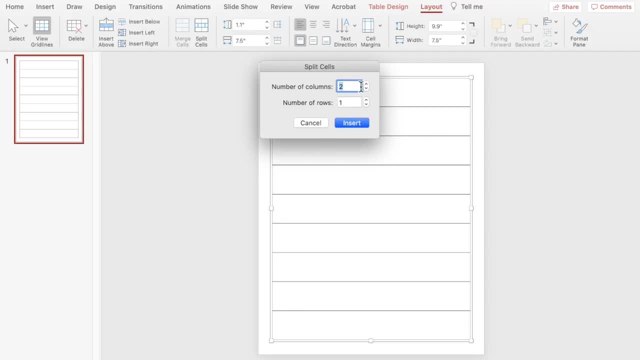 and it automatically defaults to two columns one row. And that's exactly what I want. I want the row to stay the same, but I want it to be split into two columns. So we're going to press insert And boom, you have your two columns. 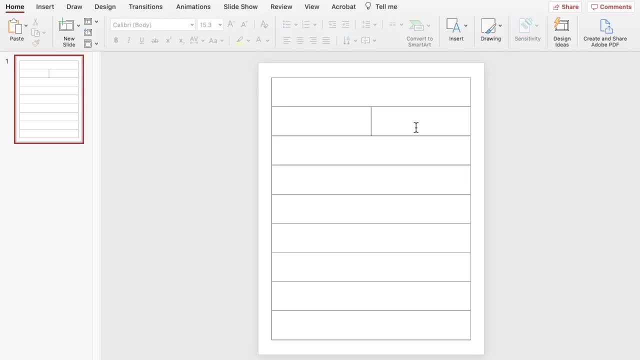 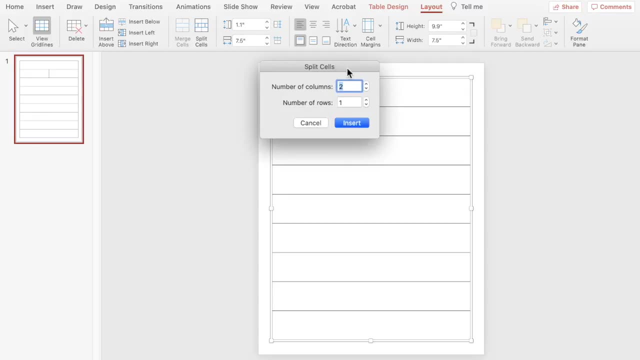 And that represents our halves, our half size, fraction strips. So now we're going to click in the third row and we're going to go to split cells. So we have that default of two columns. Now I'm going to click the arrow up to go to three columns. 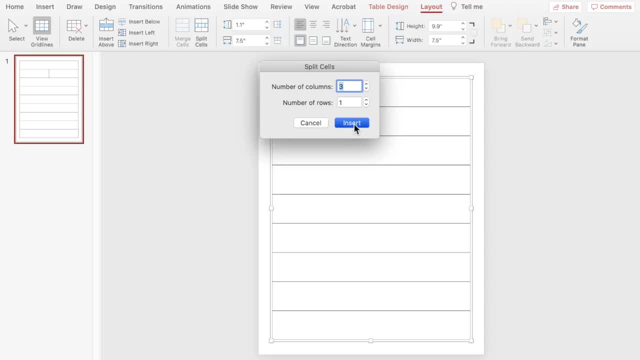 Keep the row the same. We're not changing the rows at all. Insert to three columns. So now we have our thirds. On the fourth row, we're going to do the same, Repeat these same steps. We have our fourths. 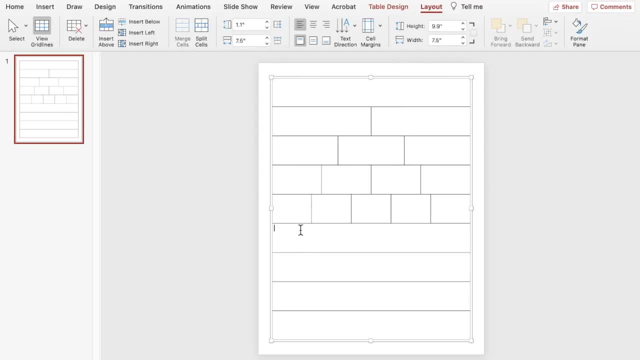 We have our fifths, Our sixths, Remember we won't have seven. Now I'm trying to click on, or I couldn't go up to eight, so I typed it in and I'm pressing insert. Sometimes I get this error message: 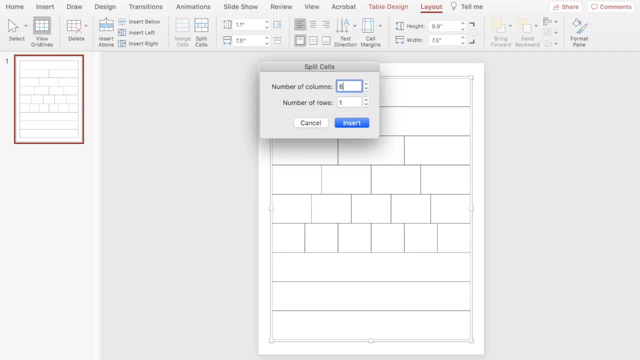 and sometimes I don't, which is interesting. But how I'm going to do this is: I'm going to go to the third row and I'm going to go to the fourth row and I'm going to go to the fifth row. 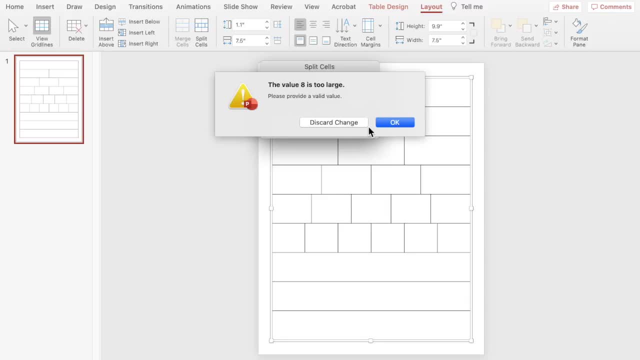 and I'm going to go to the fifth row and I'm going to go to the sixth row, but however, we can work around it. So if you get that error, remember eighths are just fourths partitioned in half. 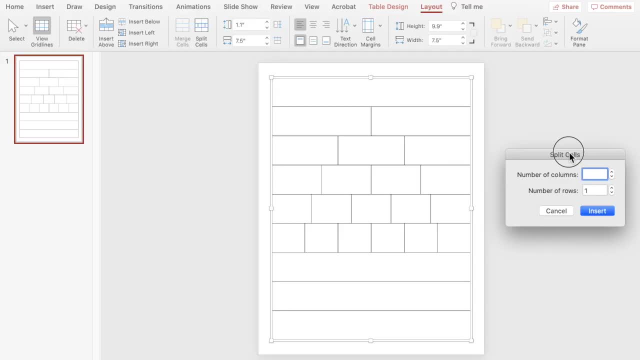 or halves partitioned two more times. So I'm just going to put four in here, and then you could have left it highlighted or highlighted again, and then I'm going to split each of those separate cells into two columns and that gives us our eighths. 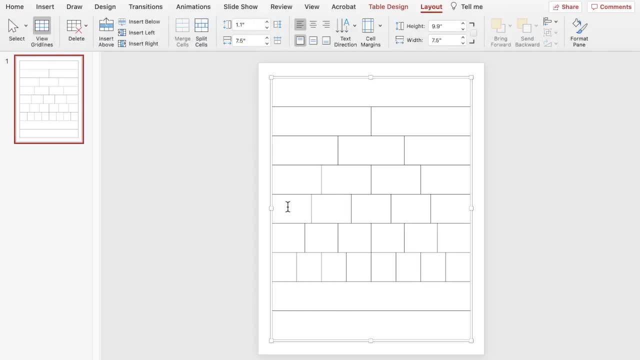 The same with the tenths, So you can also copy and paste. So if I right-click and hit copy and here click paste, I have my fifths and while it's selected, I'm going to go up to split cells. 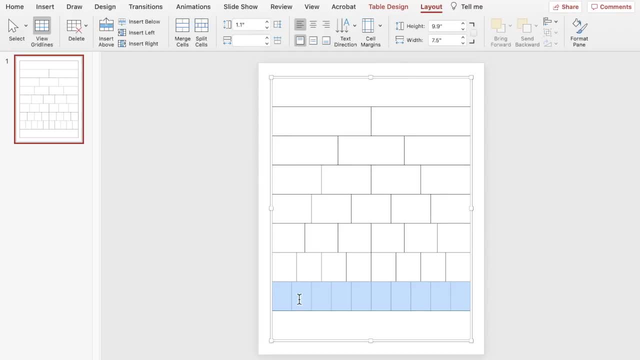 leave it at that, default two. and that creates my tenths. And then, for sixths, we're going to copy our sixths, paste them and then split them into two equal parts or two equal shares. All right, so there is your basic, basic template. 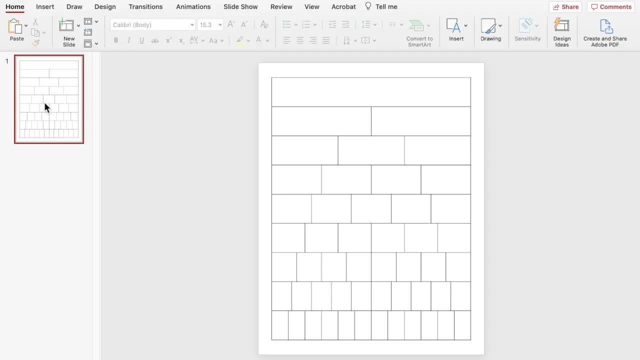 So that one we're going to absolutely leave the same. leave just like that. So you have a blank Blackline master for fraction strips with no labels. So now we are going to create our labels. So I'm going to come over here to the slide on the side. 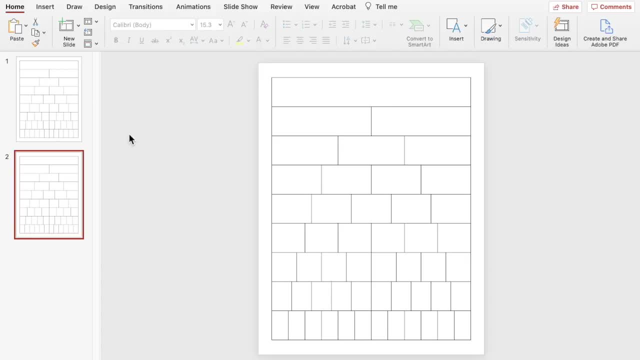 and I'm going to hit duplicate slide. You can also hit command D or control D if you have a PC, So this one. I'm going to create text boxes to add in for my fraction symbols. So let's do about this size. 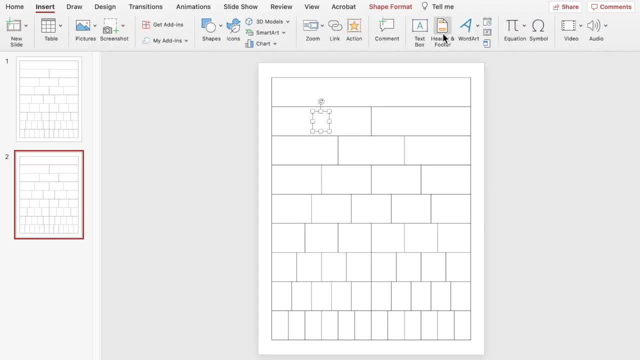 and then inside of it I'm going to come up to insert and over to equation and then hit fraction and select that first fraction. I'm going to make sure I hit in the bar: Here's one. And then on the bottom, it's two. 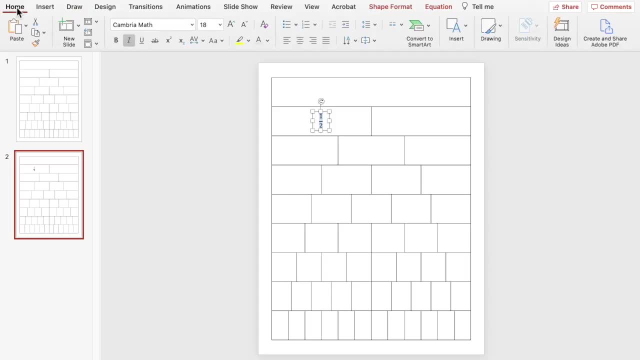 I want the text to be a little bit bigger And then center it. And there's my half. so I'm going to take that and duplicate it, To place it over here, And then I'm going to duplicate the half again, bring it down here. 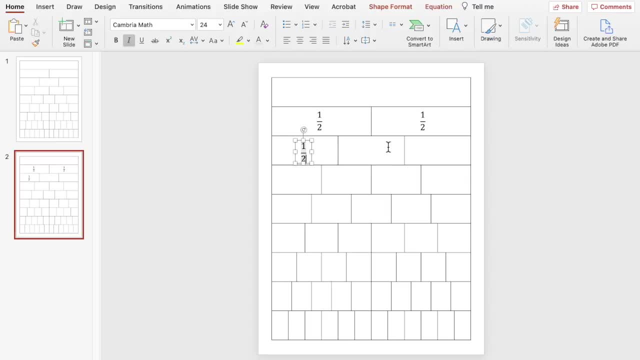 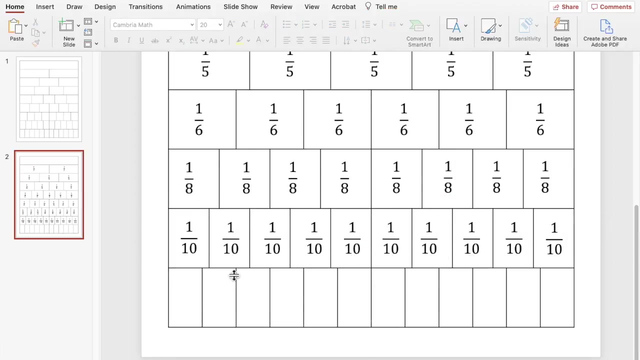 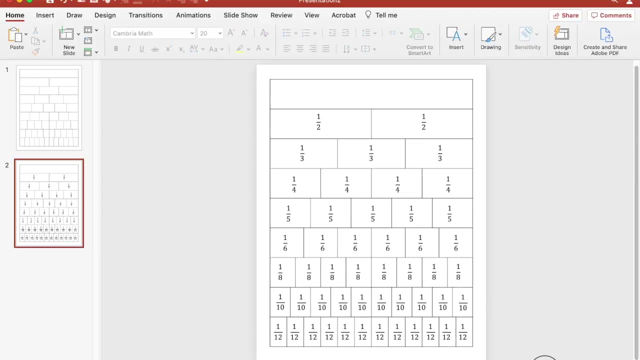 and then change the two to a three to create my one third. Let me make sure that's where I want it to be. So there we have our fraction strips. Let's add in our number one In the middle And make that a one. 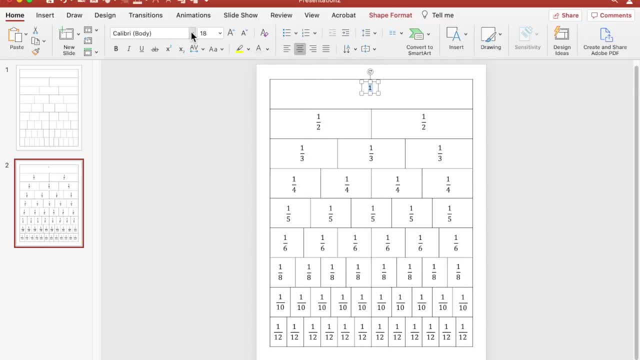 And I want that to have the same font. So it's going to be Cambria math And make it a little bit larger Because it is the whole. Alright, so there are our fraction strips, So we have our black line masters, without labels. 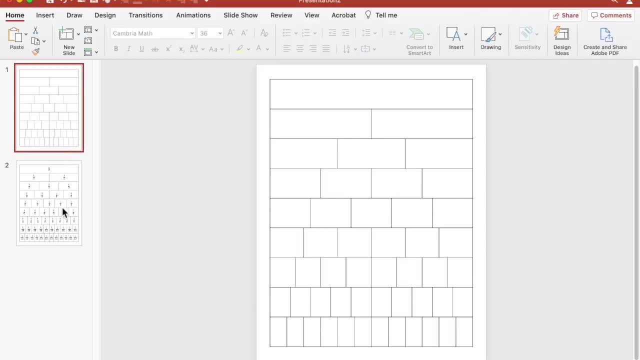 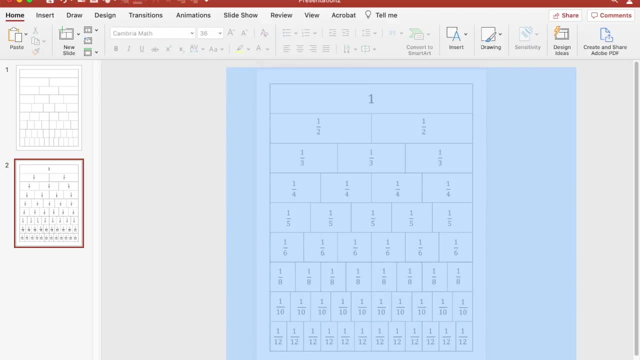 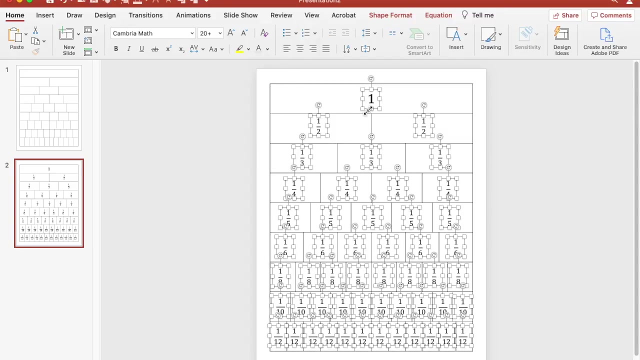 and then with labels. And now what we're going to do is add in the color. But first let me, I'm going to select all And then I'm going to hold down the command button and deselect the table And then group all of my fraction labels together. 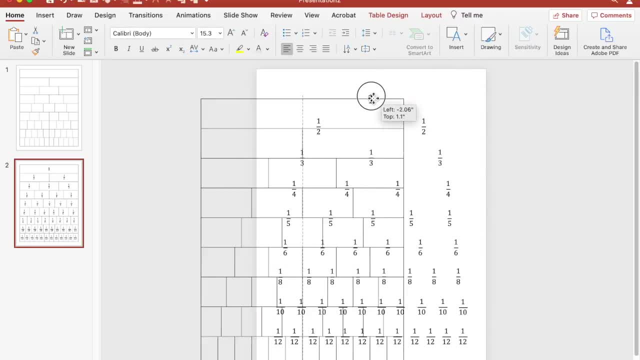 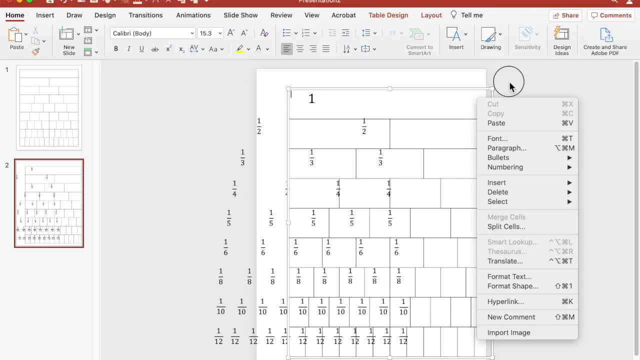 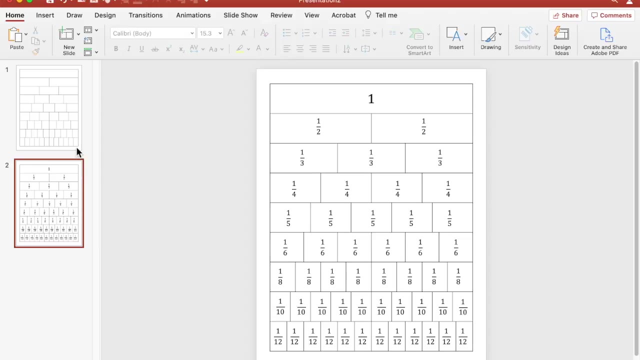 So now I can move them around if I want, But I'm going to hit undo to put them back in place. Alright, that's going to come in handy when we're adding in our color. So we're going to duplicate these two slides. 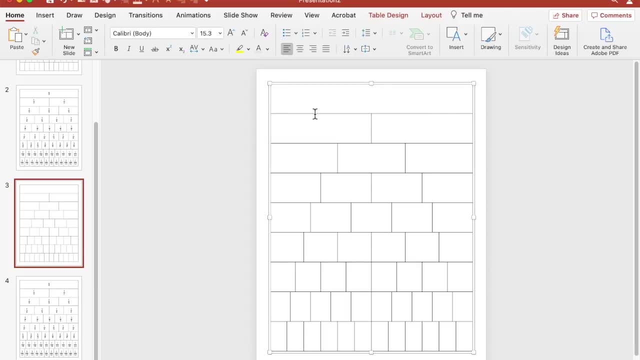 And we are going to add in our color, Our very common colors that you'll see on most fraction tiles or circles or bars. You see different colors, But generally you're going to have these main colors for the strips. So for our whole we're going to come up to table design. 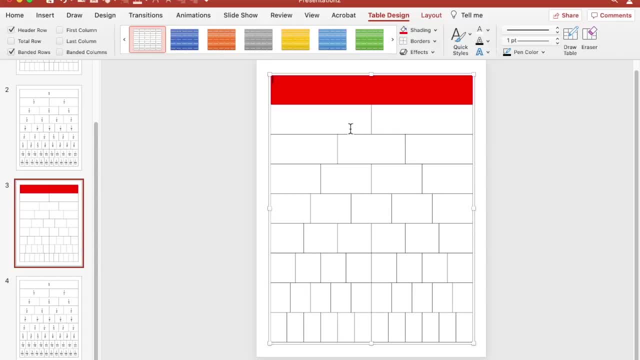 and go to shading And we're going to make that red. Our halves we're going to make like a navy blue. Our thirds we're going to make like a peach color Salmon. Our fourths are going to be yellow. 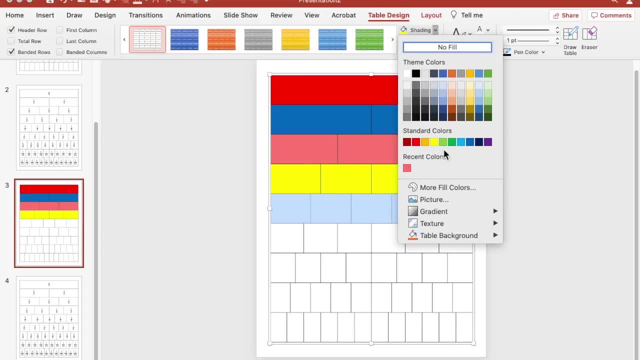 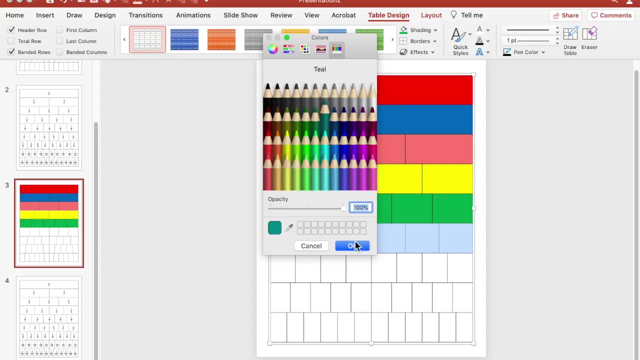 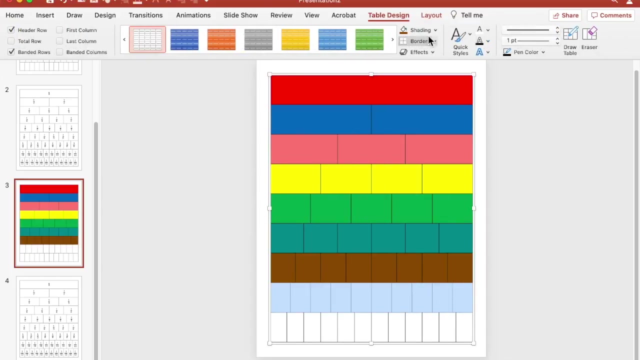 Our fifths are going to be green. Our sixths are going to be like a bluish, a teal And sky teal. There we go. Our eighths are going to be brown Mocha. Our tenths are going to be purple. 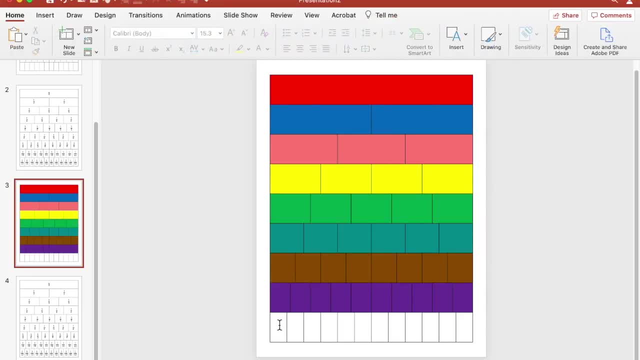 My favorite color, Purple, And then so normally you see with fraction tiles you see the twelfths in black But that you kind of can't see the lines. So I'm going to make that, You can make that white. 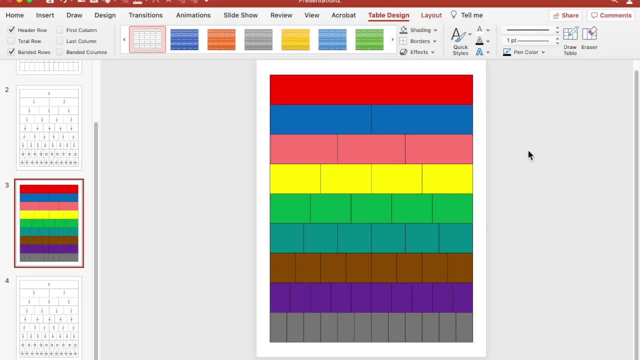 You can make them a light gray or a dark gray. So I'm going to make them a dark gray. And there are our fraction strips Without labels but that do have color. So similar: here black line And here color. 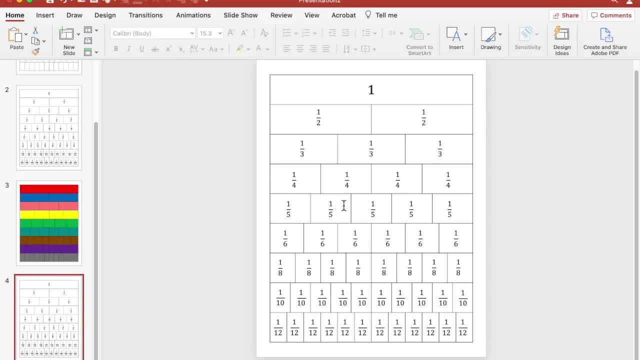 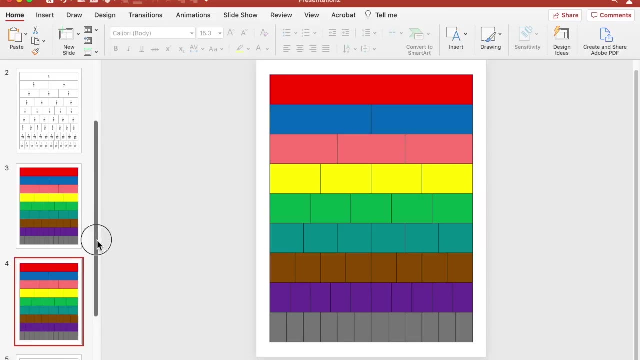 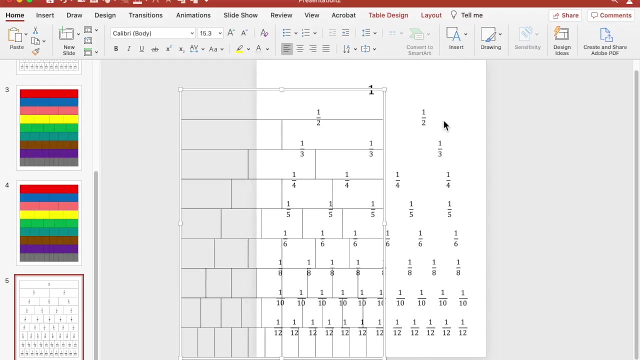 So we're going to do the same thing, But with our labels. So I was going to color them individually. But something that's even faster: Let's duplicate this slide with the color And we're going to take. Let's move the table out of the way. 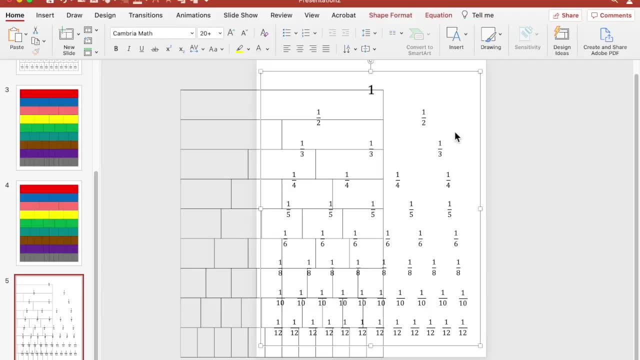 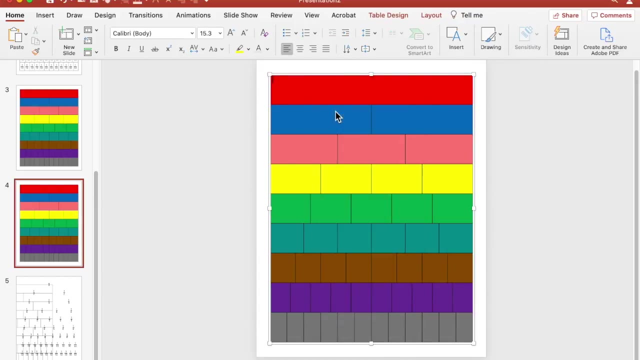 We're going to select those fraction labels that we grouped together, So now they're one unit. So if you press command C to copy or write, Click and then copy And then go back to this slide And then right click and paste. 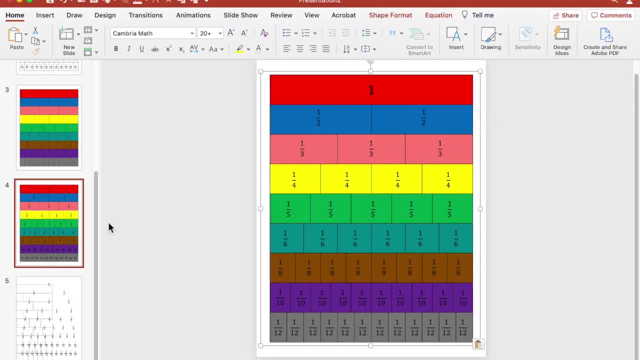 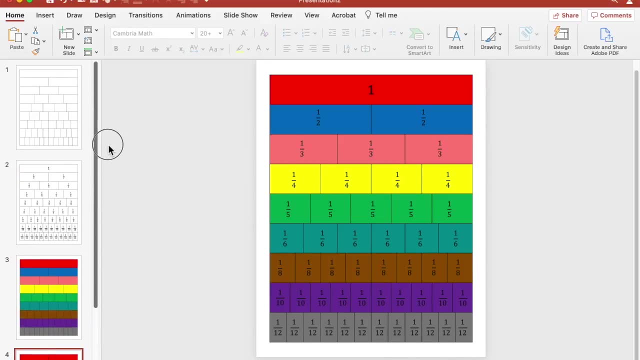 Boom, There are your fraction symbols, So we can delete this slide altogether, And there we have our fraction tiles, Or your fraction strips that you can print out yourself for your own students Or for any children that you're working with at home. 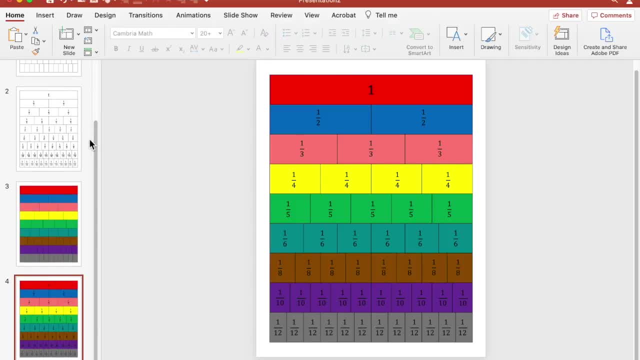 So the last thing you need to do is just save it to your computer, And it's ready for you to print. 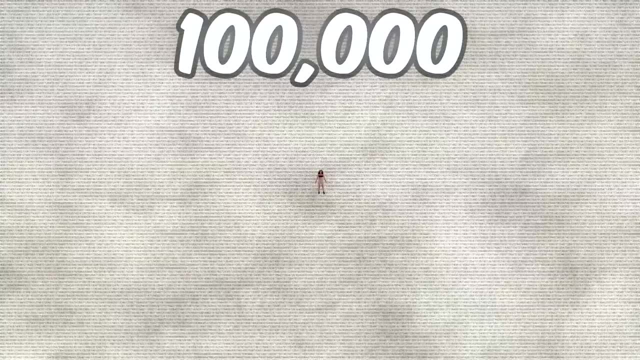 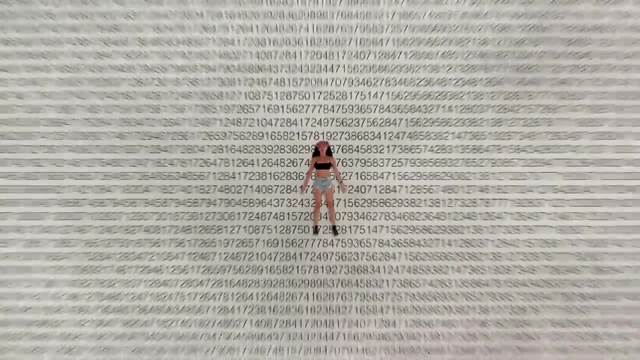 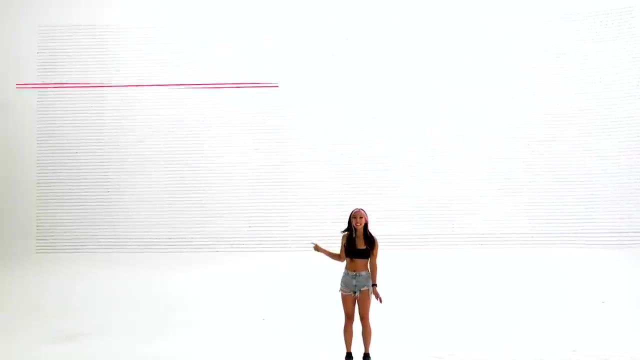 This is a 100,000 digit math problem and I'm going to spend the next 10 days attempting to solve it. This is definitely the most insane thing I've ever done. This math problem is massive. There's literally 100,000 digits on this wall. This is so tall. There is 69 and a half rows. I do not know. 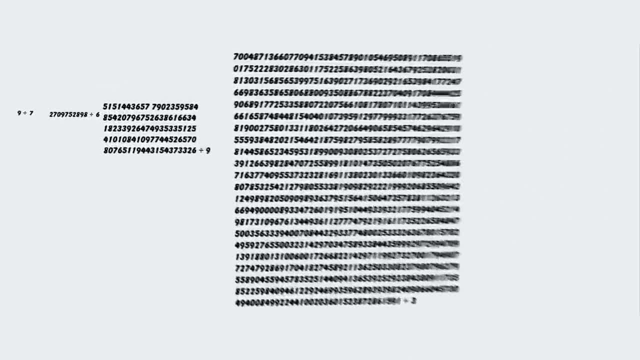 how I'm going to do this. I'm also going to be solving a 10,000 digit, 1,000 digit, 100 digit and a 10 digit math problem, But first I'm going to solve this one digit problem. Hey.